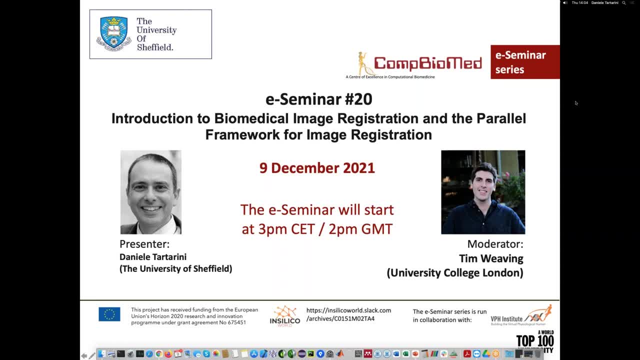 maybe even share these e-seminars with your friends and colleagues. There'll be a Q&A session at the end of the talk, so please save your questions until then. Once the talk is finished, you can post your questions in the questions tab and I will read them out to Daniele to. 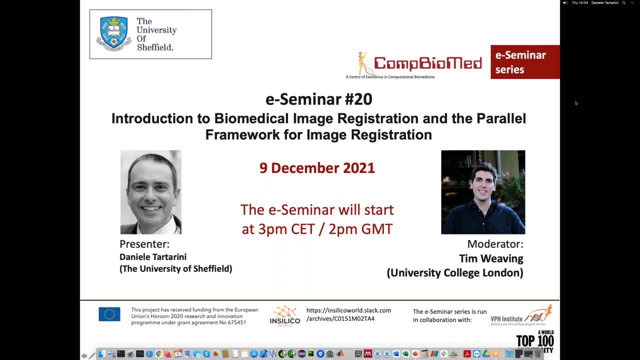 keep the session running smoothly. Now, that's everything from me. I very much hope that you enjoyed today's talk And, without further ado, I'm going to hand over to you, Daniele Hi. Hello everyone. Welcome to the bFIRE conference. 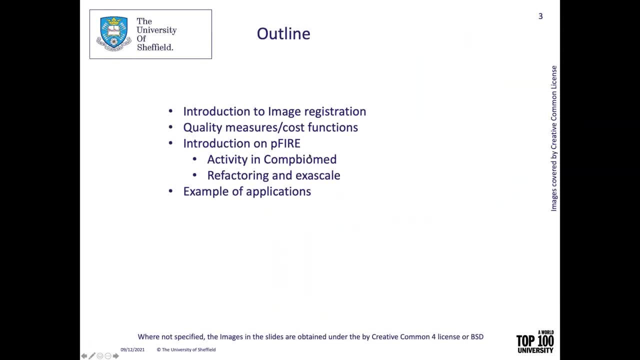 So today I'm going to introduce you the following outline in the talk. This is a talk which is part of a two talk series. The second one will be given next year. it will be in more detail than the second part of this talk, which is BFIER. So I'm going to introduce you about 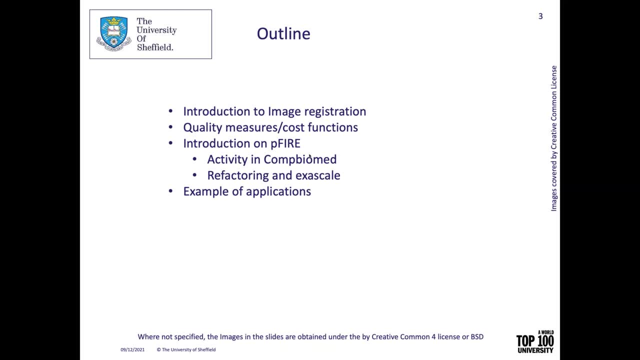 the image registration and give you an idea of the quality measures and cost function. using this process, I'm going to introduce you BFIER, the parallelep framework for image administration, and what is our effort in refactoring towards exascale. and then some. 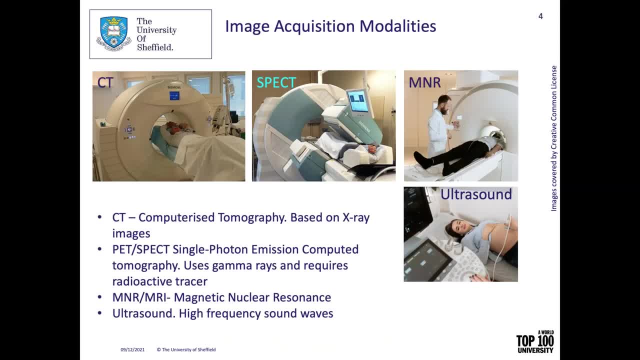 examples of applications. So image acquisition is a very powerful diagnostic tool and it's used by the doctors to investigate particular situations of the patient. So there are different technologies that can be used and they depend on which type of tissue has to be investigated. 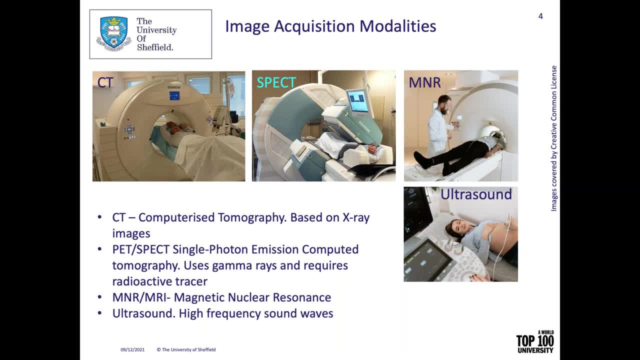 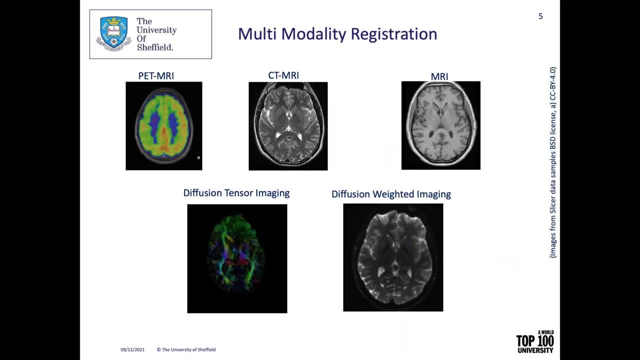 For example, bones is better investigated with the CT scan, which is based on X-ray. So there is a range of possibilities, and that depends also on the physics involved for doing the inspection. So these technologies can produce different types of images, For example MRI images. these are the images of the brain and they're taken with different 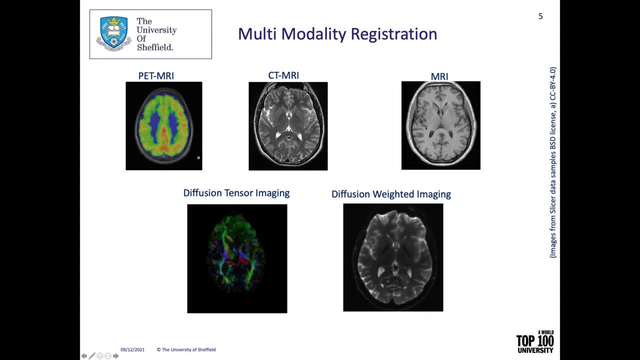 methodologies and technologies. So the MRI is a scan of a magnetic lens. So the MRI is a scan of a magnetic resonance and precision-emission MRI- it's another image generated which explains the function of the brain. So when we analyze these images, we have a multi-modality number of images which can. 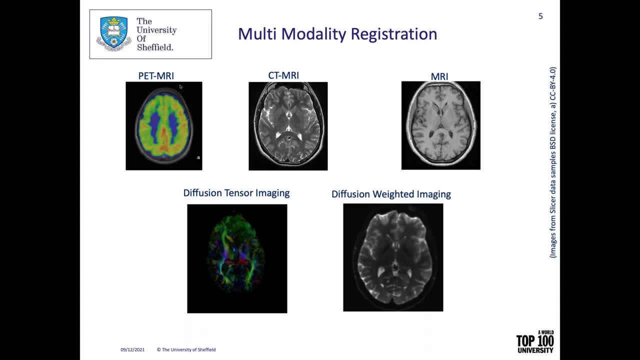 highlight different functionalities of the brain, different information in the brain. Currently the machines. Okay, So we have a couple different technologies together. For example, this image is obtained coupling the CT scan with the MRI in the same machine. It was not always the case and in the past you had to have a scan in one machine and 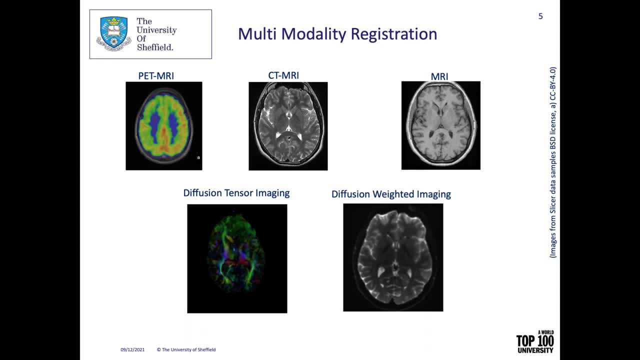 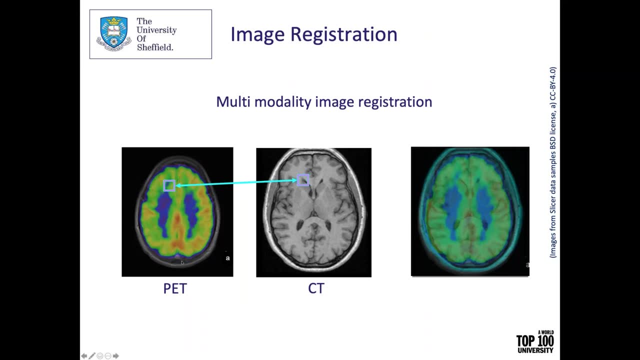 then another one, And then the two images need to be overlapped in some way to get the same information. Image registration can be used exactly for this purpose. So let's say you have two images. Let's say you have a precision-emission image and a CT scan and you want to see what happens. 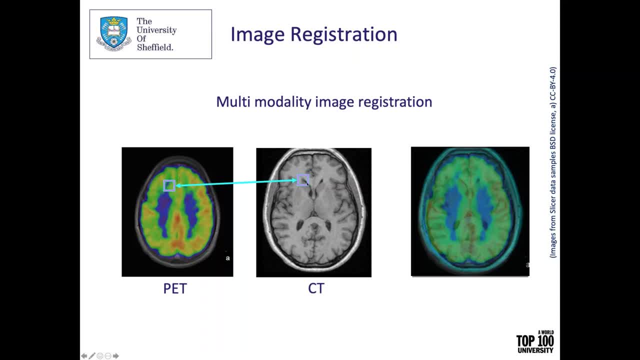 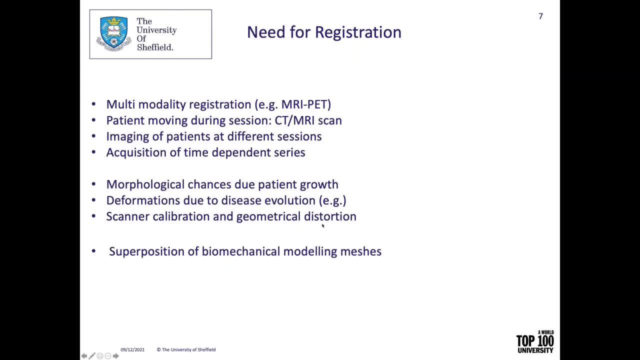 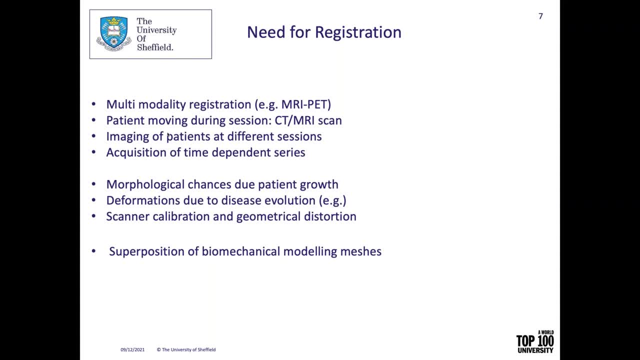 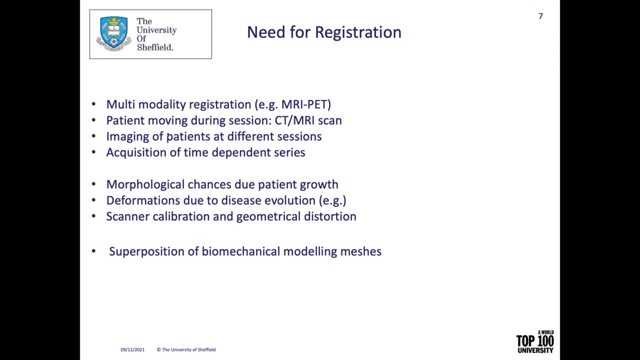 another modality and the two images are not aligned. So to analyze the two images you need to overlap them. It's also possible that you do a time-variant analysis. It means that you acquire images Different time steps, So when you do that there could be movement inside the image. 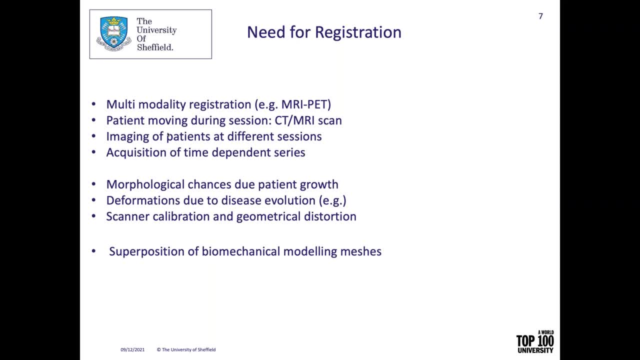 So you don't have good information if you don't register, if you don't overlap correctly the two images. It is also the case that the patient develops some disease, some lump, that they grow and you want to see the evolution of this disease in time. so all the images captured need to. 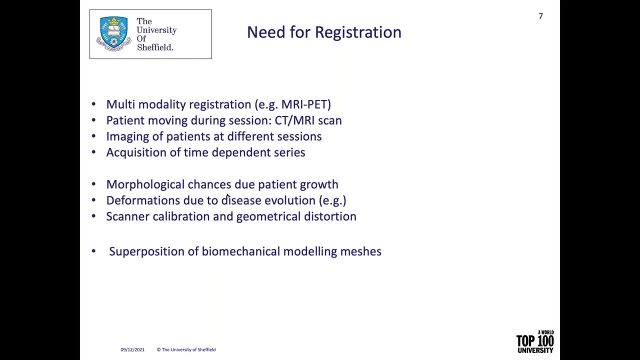 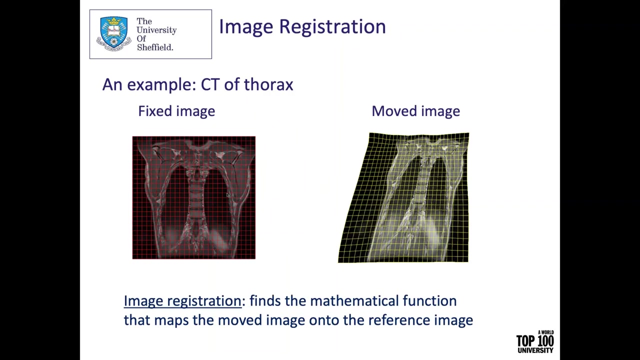 be aligned properly. Also, there could be problems in the scanner that can generate some geometrical distortion and some problem calibration. Last but not least, you can use the registration to overlap some modeling technique like meshing of some part of the organs. 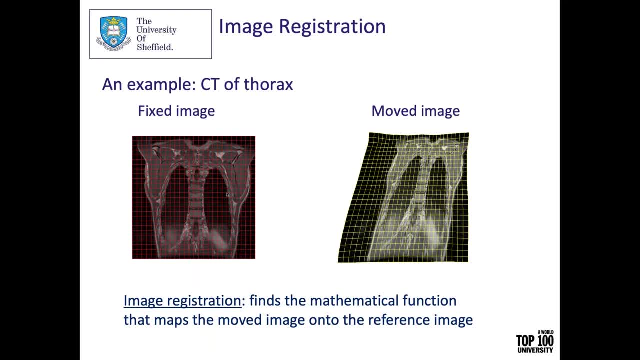 Let's see an example On the left. This is a CT scan of the thorax and this is an image which is taken as a reference from the patient. Then assume that you have another image where the patient moved for some reason. and now, 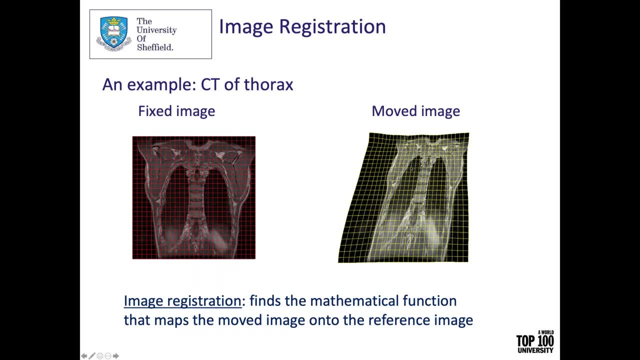 you cannot compare what happened in the two images, because if you overlap these two images, you are not able to match the different region. So what image registration does? Instead, you find a mapping function that allows you to take a moved image and overlap it to the reference image. 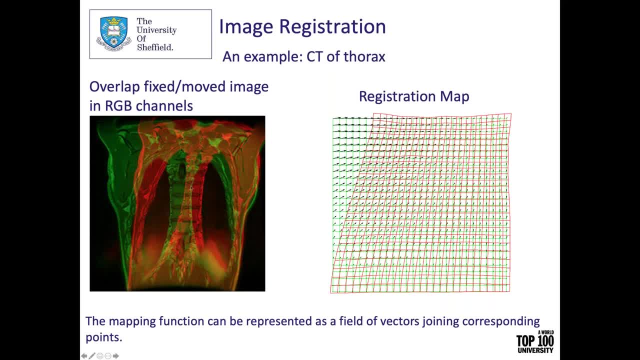 The problem can be seen another way. So if you plot the two images into different color channels, you can see in green the fixed image and the moved image. Is this correct? Yes, Clearly, you are not able to compare the different parts of the image because they are not overlapped. 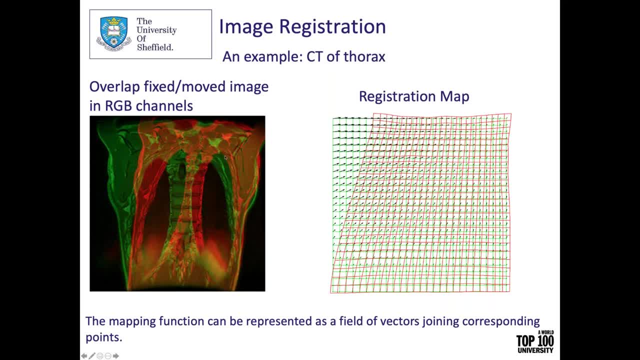 correctly. So you need to convert. you need to morph the second image on the first one to compare properly the different areas in the image. If you look on the right, the function that makes this can be seen on a map in a mesh. 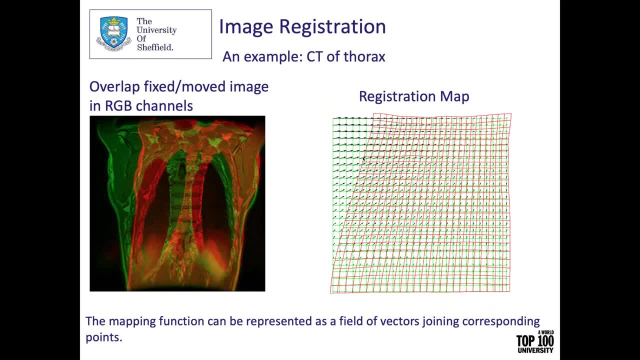 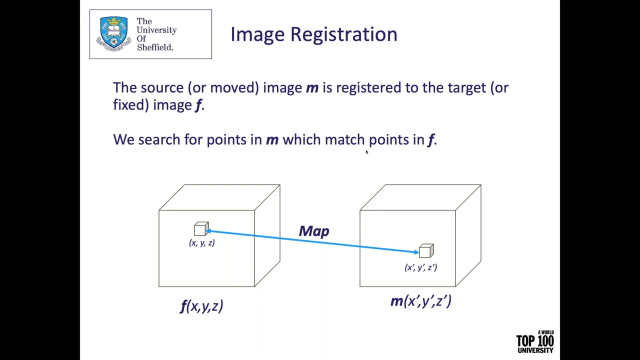 If you remember the previous slides, they were overlapped on these slides in a mesh, So the arrows you can see in this plot are exactly the displacement that allows you to map one image on the other one. If we generalize the problem, this can be applied in 3D and you can have a 3D volume. of the image. If we generalize the problem, this can be applied in 3D and you can have a 3D volume of the image. If we generalize the problem, this can be applied in 3D and you can have a 3D volume. 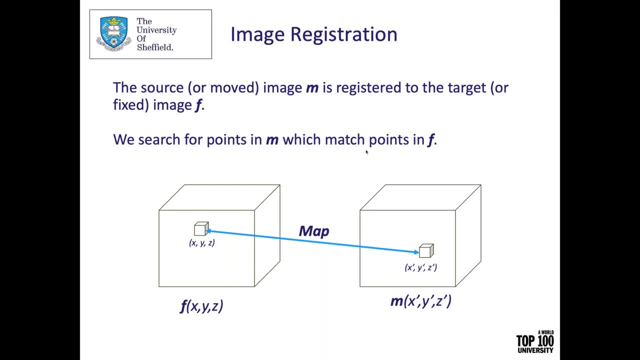 of the image And you need to find in the same way the mapping function that allows you to put in relation the coordinate at one point, one voxel in one image to the other voxel in the other image. So if you think the image is just a function which says which is the intensity value of 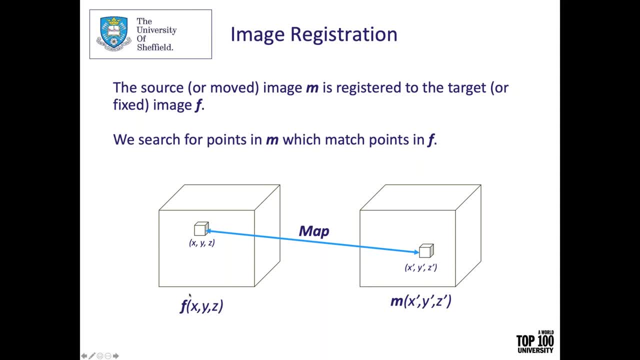 the image in that point. So F&M are two functions that say what is the intensity of the field in that point. So let's call the x, y, z, the coordinate of the voxel in the fixed image, and x prime, y prime, z prime, the coordinate of the voxel in the moved image. 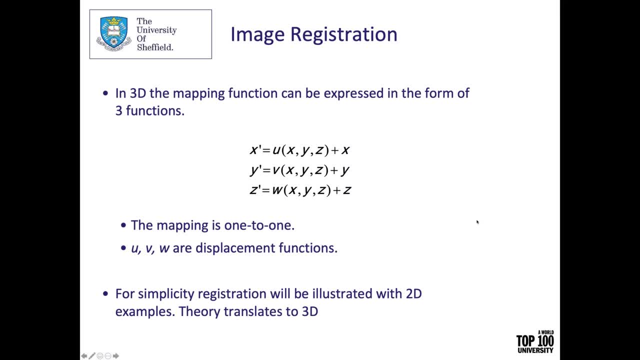 We can write the equation of the translational coordinate considering the x prime, y prime and z prime are just the original coordinate plus some values. These values are the displacement, So the mapping is one-to-one. What we need to find to register these two images? 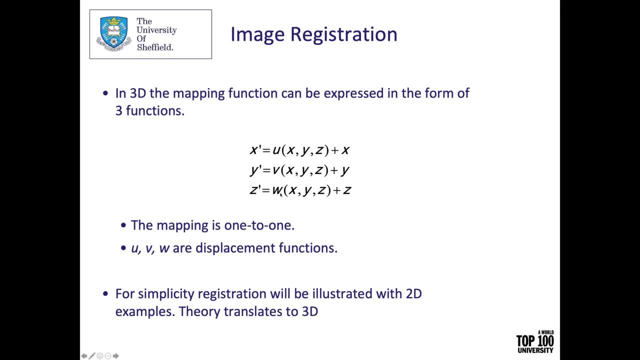 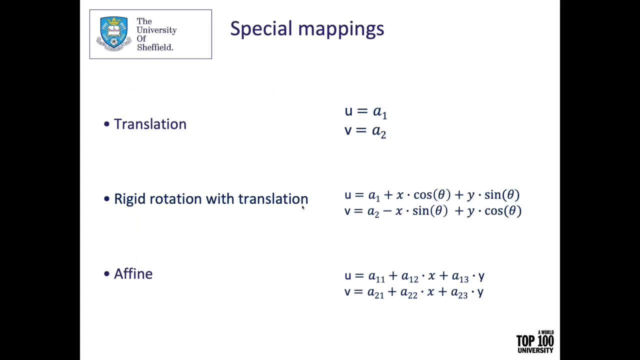 are the values u, v and w. For simplicity, we will discuss only about 2D images, but it applies correctly. We can refer easily to the 3D case. So the most simple mappings that we can have is the translation. 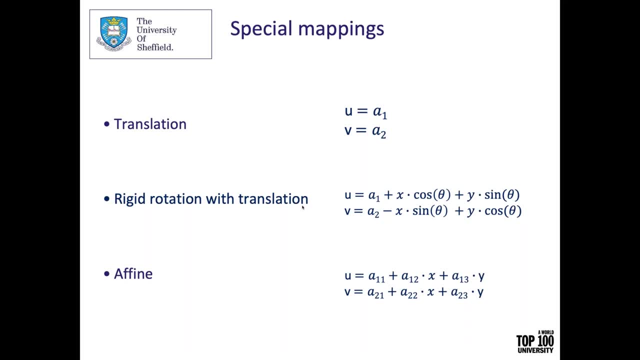 So one image is just the translation of the other one. So what changes is just the addition of some constant. One image can be rotated and translated with respect to the other one. so we have a component of the translation plus the translation, plus the rotation. 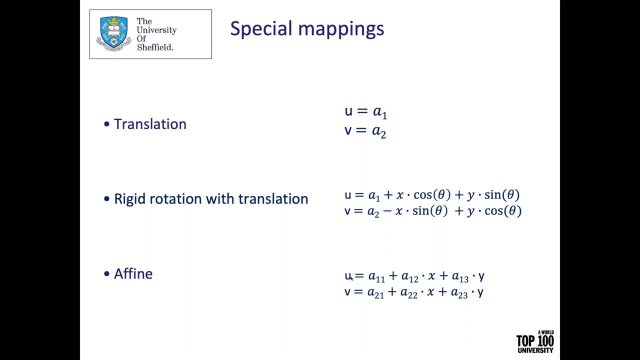 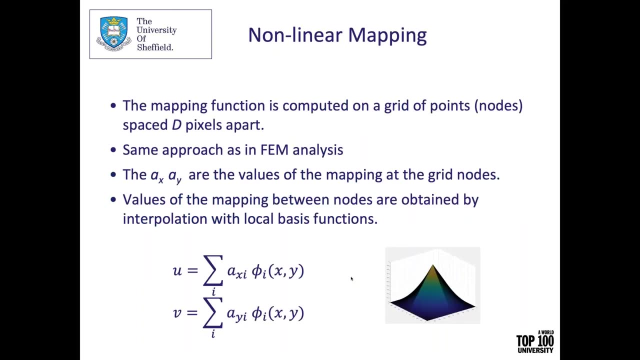 or we can have an affine transformation, which is we can imagine the course of the frame of the image, which is the example of this t-thorax I showed before. The most interesting thing case is when we use nonlinear mapping. 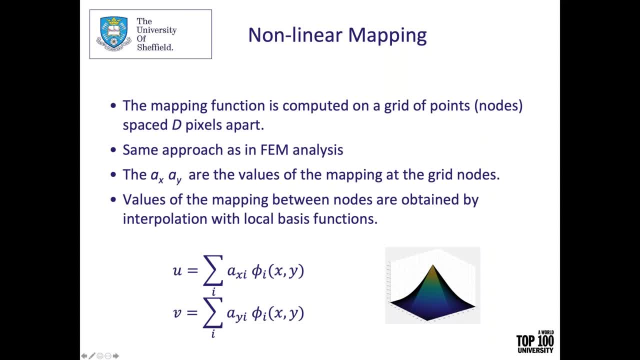 So we leave the freedom to u and v to assume any possibility, any type of function. This is quite similar, the proto-infinite element to find the displacement when we apply some force to an object. So, as usual, to find this function, you imagine to discretize the domain. so you apply a mesh and then you want to identify what are the basis functions identified on the nodes, on the mesh. 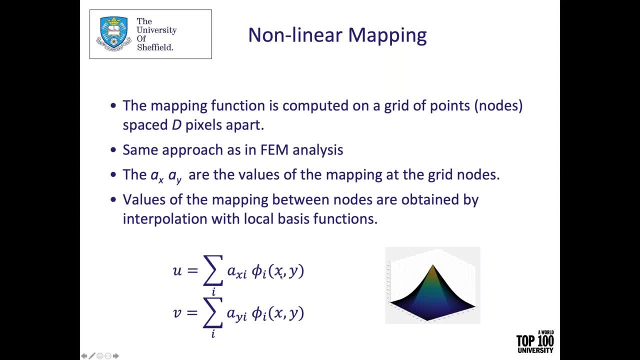 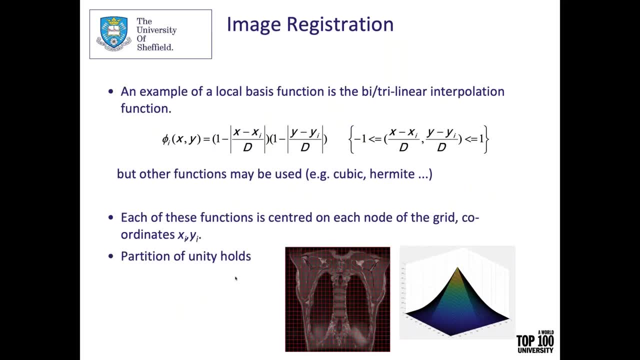 So in this case, this placement along the X is given by a linear combination of the basis function multiplied by a value, which is the degree of freedom. We can apply a different type of basis function. Usually they're polynomial. It could be three, or bilinear or trilinear polynomial, depending if you're in 2D or 3D. 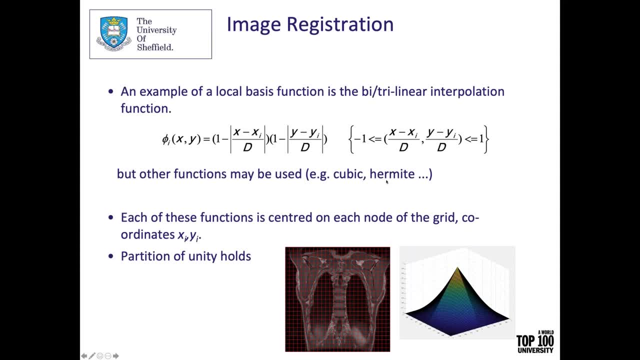 It can be cubic, the order of the polynomial cubic or might polynomial, There are different possibilities you can use. So each function is centered, each basis function is centered on the node, on each node of the mesh and the concept of partition of units also. 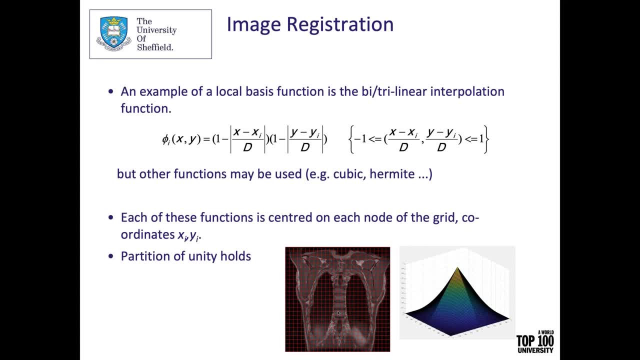 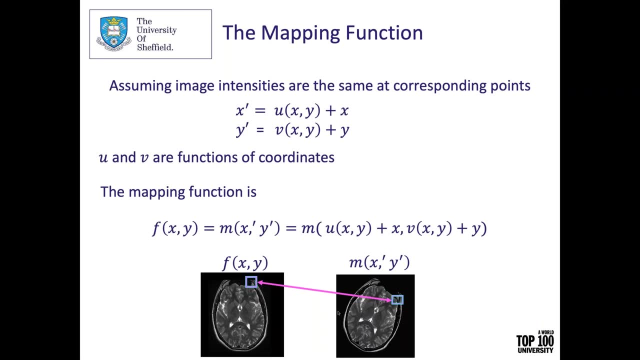 So it's one in the node and then it's zero in the neighbor nodes. So again in 2D, the displacement allowed to put in relation the value of the images into corresponding pixel onto corresponding voxels. So these two functions, this placement, are functions of the coordinates. 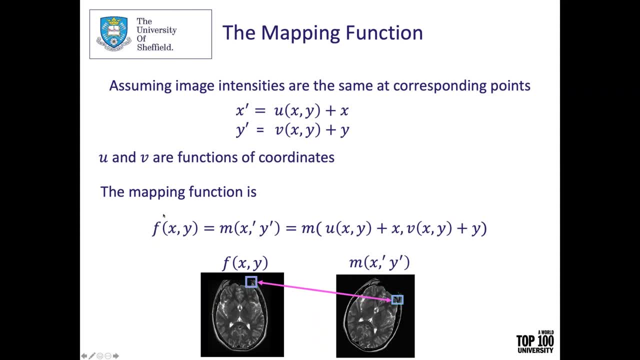 So if we write an equation, we add that the fixed image has the same value As the moved image computed in the X prime and Y prime. So this is the fixed image on the left. This pixel here which is magnified just for example, has the same value as this pixel here in the moved image, just considering the function maps, the two coordinates. 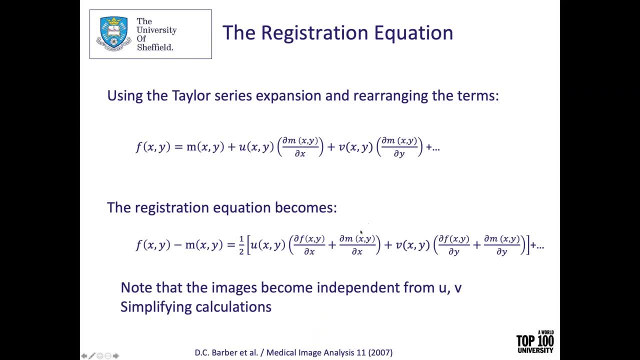 Now we want to simplify things or complicate them in some way We can express, we can expand this equation using material series. So you have the equation and then this expansion theory of series. you recognize the derivative and the u and d functions. then there will be higher order terms which are ignored and they will have an impact, and we'll see later. 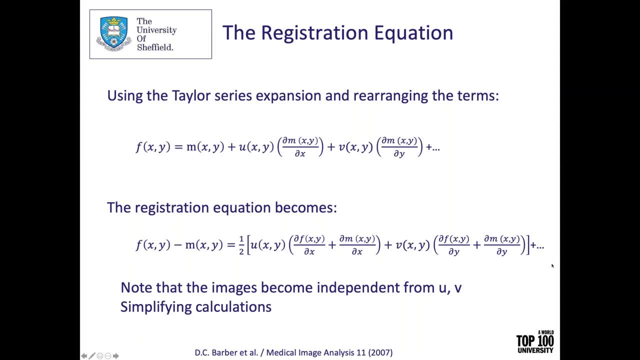 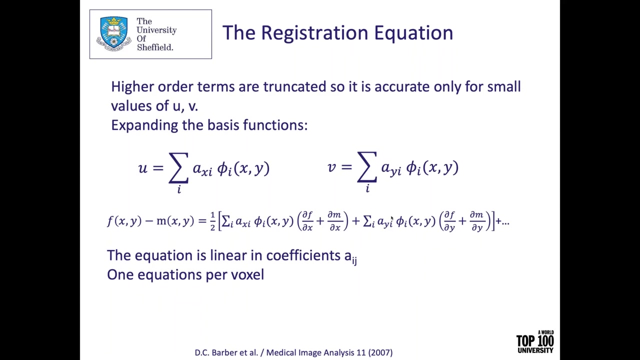 So the registration equation becomes the following one: The important thing is that you will notice that the u and d functions now, due to the derivative, are outside of the m function, So this simplifies the solution of the problem. Clearly, as we apply the finite element method, we need to express the displacement as a linear combination of the basis functions. 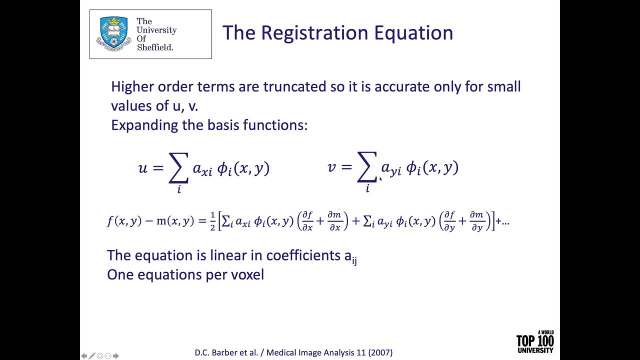 So degrees of freedom A and B, And with respect to x and with respect to y, and the displacement function u and d. So the registration equation becomes again as before, but we're just expressing explicitly the degrees of freedom. So there will be one equation for each voxel or each pixel of the image. 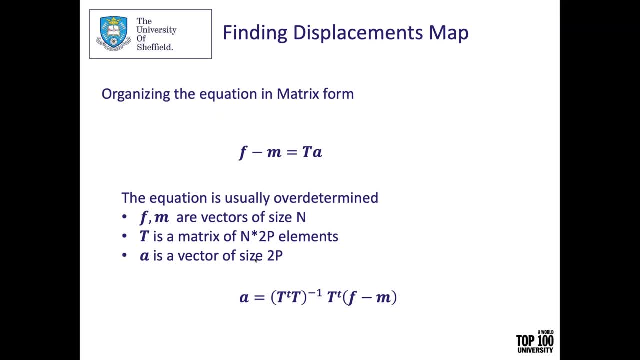 Then we have the. we can express everything in a matrix format And usually this equation is overdetermined. So there are more values of truth with respect to the degrees of freedom And we can solve as usual way: inverting the matrix. And the solution of the displacement is the following: 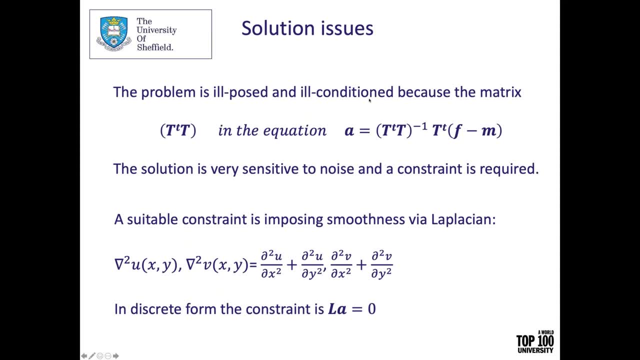 What is important is that this problem is ill-posed and conditioned. The reason is that the t transpose matrix times t is almost almost always singular. it means that this solution is sensitive to noise, which means that noise introduced in the image can generate different solutions. so to solve this problem as usual can be used another constraint and the way to go. 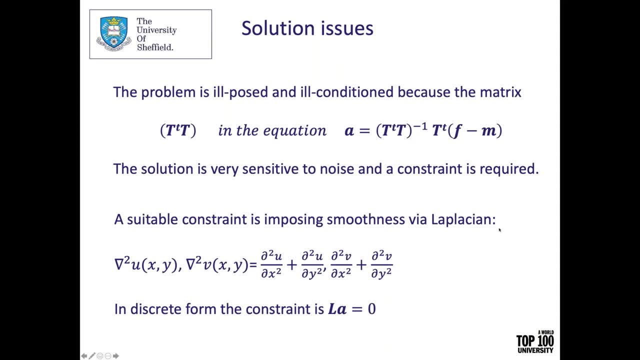 usually is to use a laplacian to impose the smoothness so the laplacian can think about the second derivative. this becomes in the discrete form, comes in discrete form with a constraint: l laplacian matrix multiplied by the degrees of freedom. the new formulation we arrive is the: 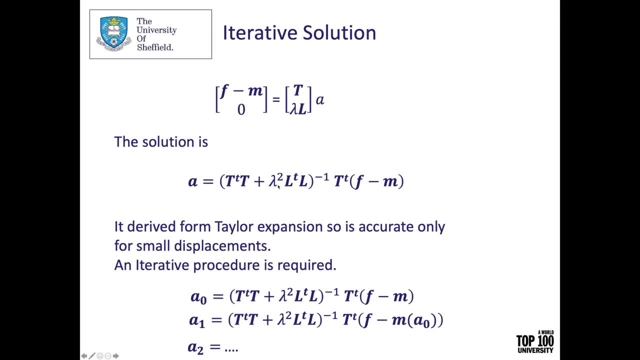 following one and we can solve with respect to the degrees of freedom. and clearly, since we expanded the equation in tillers with a tiller series, we need- and this is accurate- only for small displacement, so when displacement are larger there will be more error. that would be. 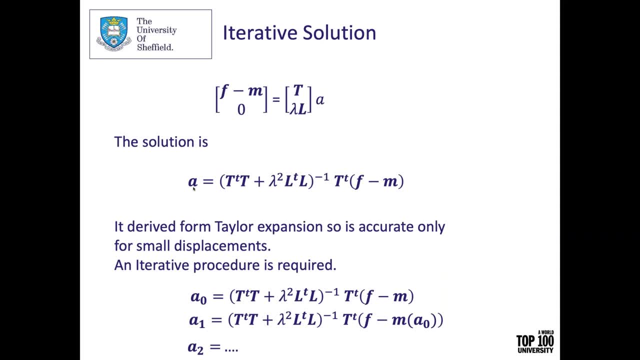 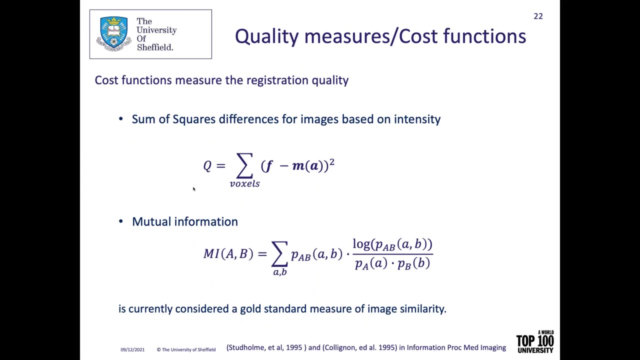 we come back to the posiness of the problem. so an iterative solution is applied and, as always when we have iterative solution, we need to find the stopping criteria when we say that we are okay with the accuracy of the solution. so there are two different types of cost function quality measures to be can be used. the first one is the more intuitive. 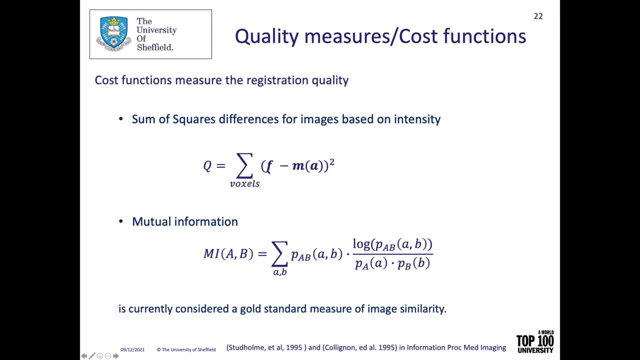 the sum of square differences. so, basically, you compute the sum of the square over the difference between the fixed image and the moved image in the same point, in the same, in the corresponding- sorry, in the corresponding- coordinate. another measure is the mutual information. mutual information is a concept that comes from the 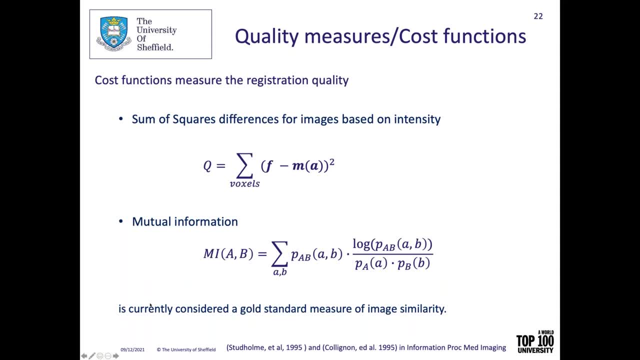 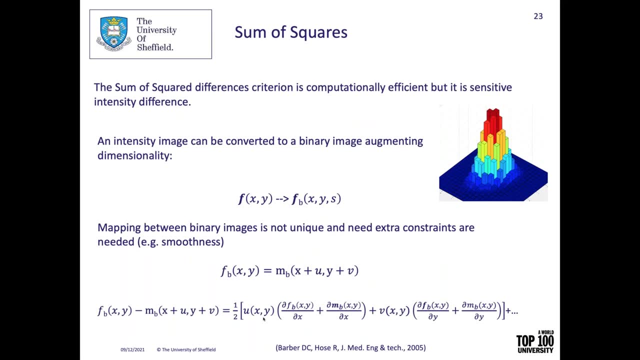 information theory and is considering a golden standard for measure of an image similarity. the problem with the first approach is that it is computationally efficient but is sensitive with respect to the intensity different in the image. if you want to interpret qualitatively this concept is that you can have the same image with two different level of gray. but 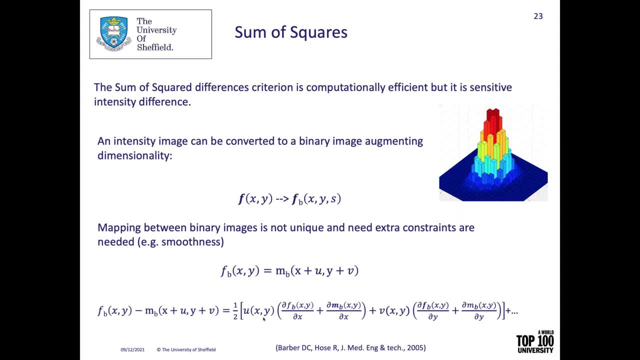 the same content. if you compute the difference between the two images, you will have a value instead of having zero. so just changing the the maximum of the degree level, you will have an error. so one solution for this problem is to use the binary image. as particular case of binary image, you will find the described in: 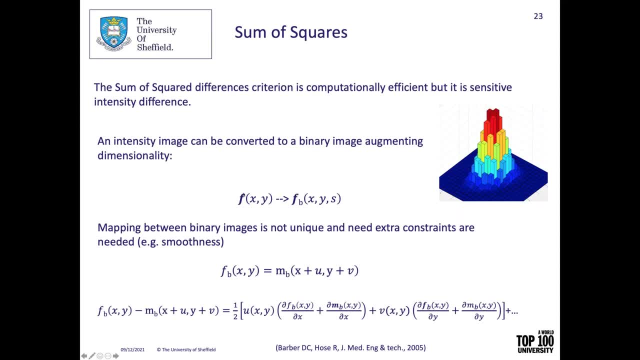 the paper of rod, function 3d, you will have a surface. the binary image, instead of having a surface, will have a stack of value that till reaching the surface. so in this plot, imagine that this is a. it is a gossam function and this has been the corresponding binary image. 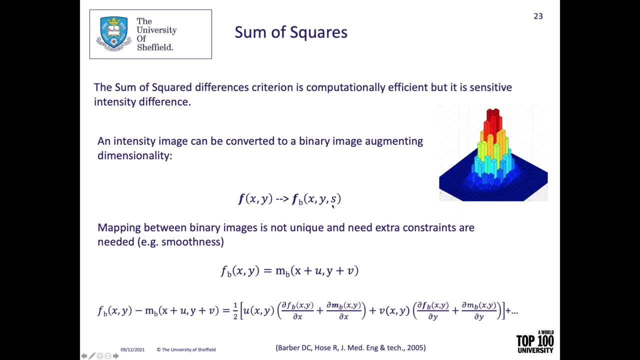 so this binary image, you will have a third coordinate, which is the intensity. but the intensity is particular, is not the value of the intensity, but is a stack of value equal to one till the actual value of the function. we're not going to detail with this approach. this requires: 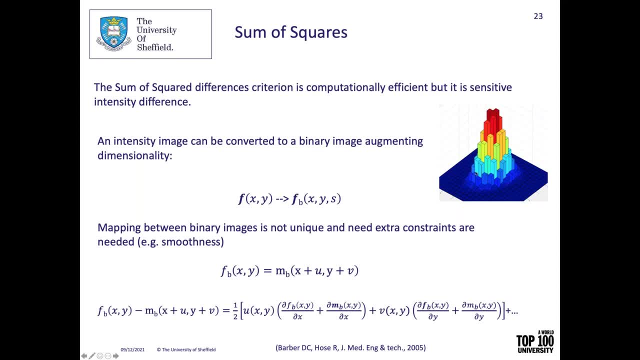 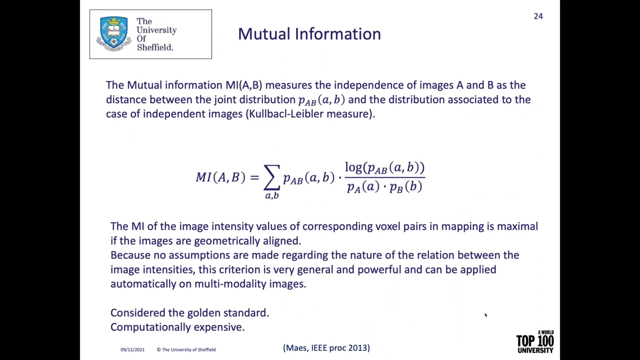 anyway, another constraint, and it has to be right. you need to have a smoothness, you have to impose smoothness on this image such that you can have a unique solution in this. with this problem, the equation- registration equation- becomes the following one, but we will not go into in detail. we will consider parliamentary interest, the mutual information, so the other. 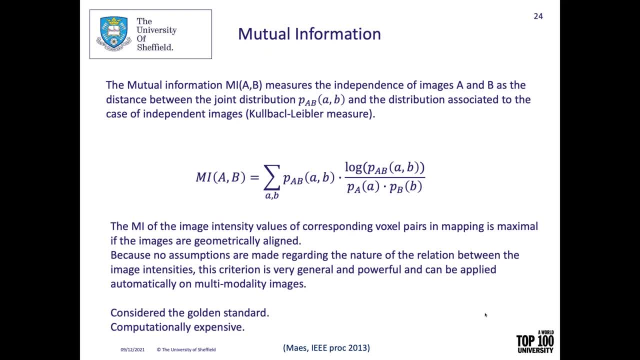 criteria is mutual information. this is the measure of independence of image a versus image b, considered as the instance between the joint distribution of the legend distribution and distribution associated to the case of independent image. this formulation is from kulak leveler and is the formula as shown before. so is the sum of a and b are gray values: intensity values. 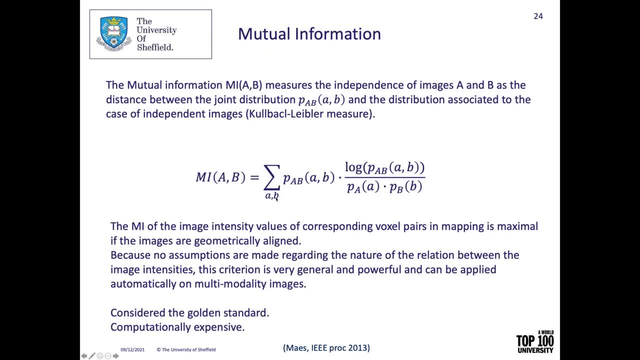 in the image a. intensity value on the image b, pa of pab is the joint uh distribution of these two values and this comes from the information theory. you will recall some of your growing eyes, the formulation of the, the entropy. but this is a will not go in too much detail about that. so, considering the intensity values in corresponding 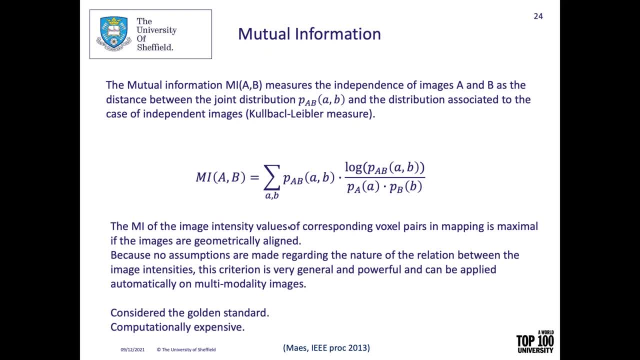 voxel pairs. the mapping is maximum when the image are geometrically online. we'll see later an example, so will be easy to understand. so the power of this formulation is that there is no assumption regarding the national relationship between the image intensities, so this can be applied for. 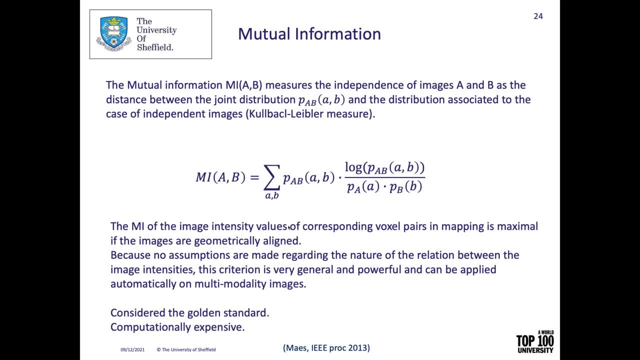 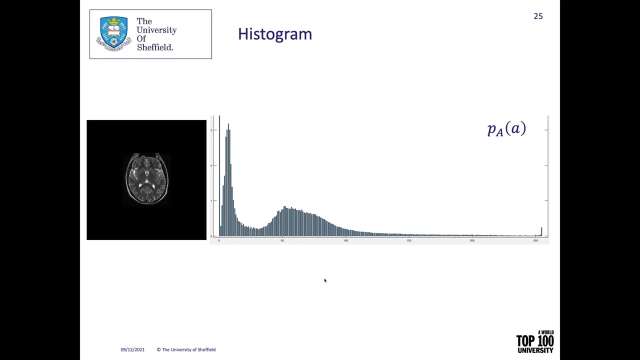 example, in multi-modality images. um, when, when you have an image in colors that uh shows the functionality of the brain, for example, another ct scan, and you want to register the two images, this approach is considered golden standard. but this is a computationally very expensive. so what we are talking, in the concept, in the formula we showed just now, now we are going to view. 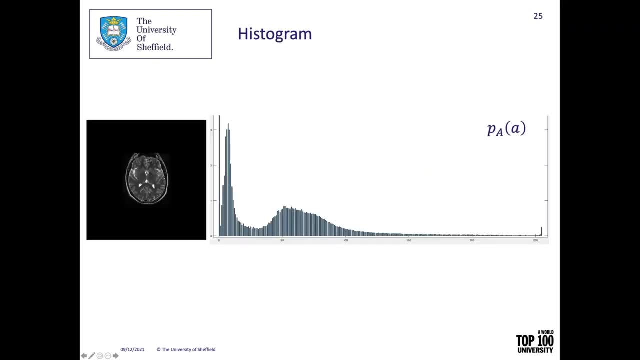 what is the meaning on these values? so if you take an image and you plot the histogram on, the image you will have in this case is a 8-bit image in gray scale, so the values are between 0 and 256.. so this histogram shows: 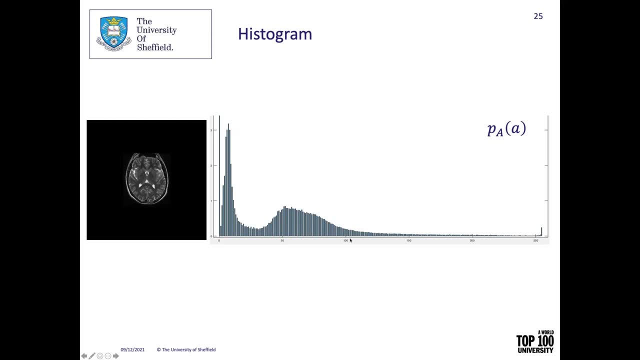 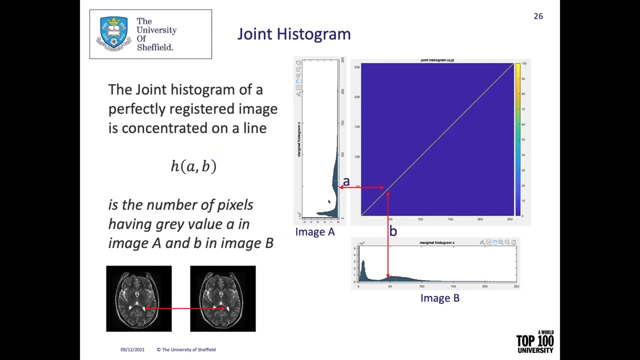 the, the count of the number of values for each gray value. so the probability of having gray value a for the image a is given by the of this histogram. What is the joint histogram? So let's start considering these two images on the bottom. If you overlap them, you will have one pixel corresponding to one pixel. 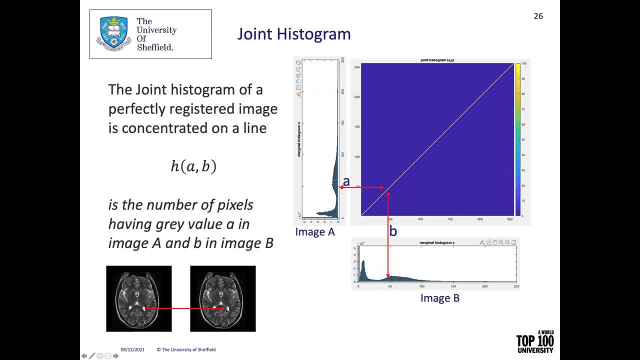 of an image, let's say this one corresponding to the other pixel in this other image. These two pixels will have two different gray values. So what is the histogram of all these couple of gray values? So, if you count all the different couples of gray values associated on the two, 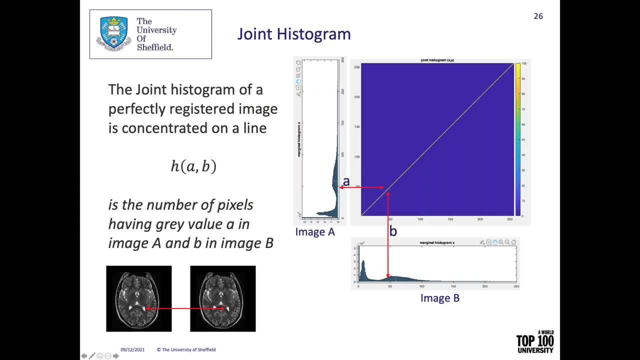 image of a laptop, what you will have, the joint histogram. So, for example, is if the image a- this is Instagram image a- the value, the gray value, a, is associated on the other image B to the gray value. 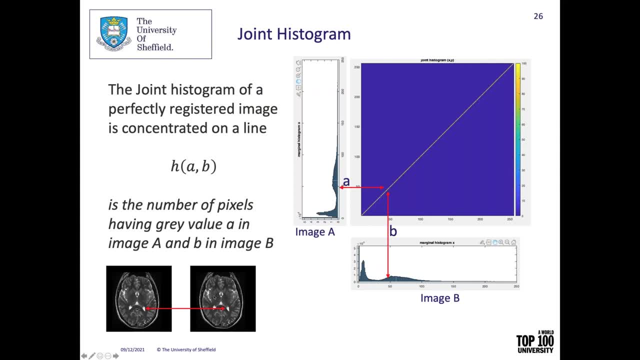 So in this case, where the two images are identical, so that is the same image, so if you overlap them, they're already registered. so it's the best possible case. You will have the same number, the same distribution in the histogram, so the joint histogram will. 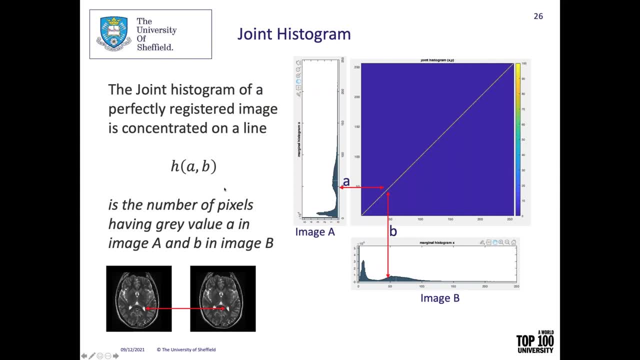 be along the line. So, if you imagine that you want to register two images, this is the best scenario. So the two images, when they are perfectly registered, the joint histogram will be aligned. But, as you can imagine, this is not always the case. 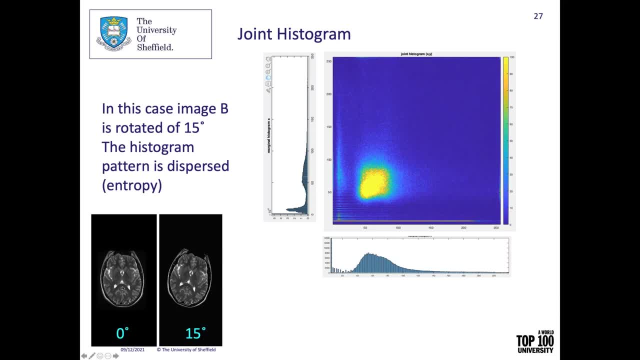 So let's assume an example. let's see an example where we have the MRS scan as a reference And another, the same MRS scan, rotated by 15 degrees. So what will happen is that the point will not correspond exactly the one to the other. 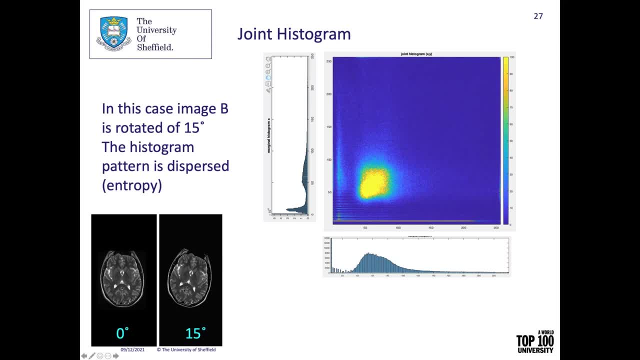 So this white here will not correspond anymore to this white here. So if you overlap the two images it will be another gray. So if you look at the image, there will not be anymore the lines, the straight line, which is to say one value with the exact same value on the other image. 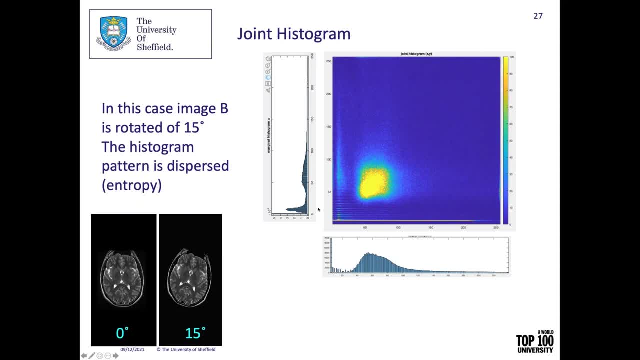 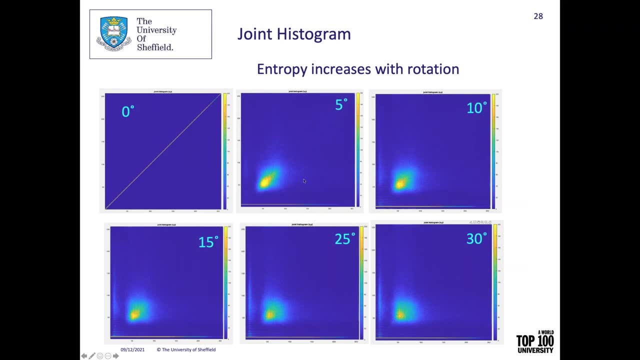 But you will have a distribution of values. The more you complicate the thing, the more you rotate the image, The more the mapping between the two images will not be aligned. So you are adding entropy to the image. You will see that the more you rotate the image, the more the entropy around the diagonal. 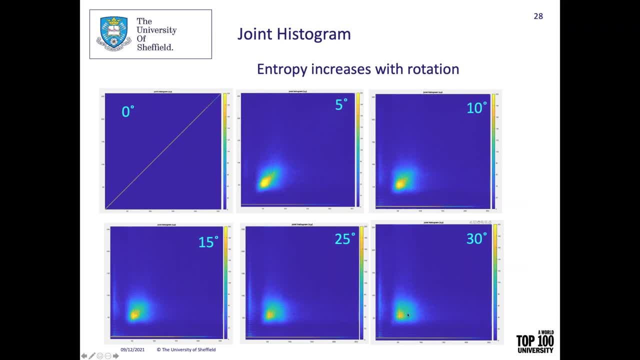 line augment So you will see that the different value distributes more around. So if you inverted the process- You imagine you want to register these two images, You will know that they are not registered. But if you, This was This is easier to simplify here. 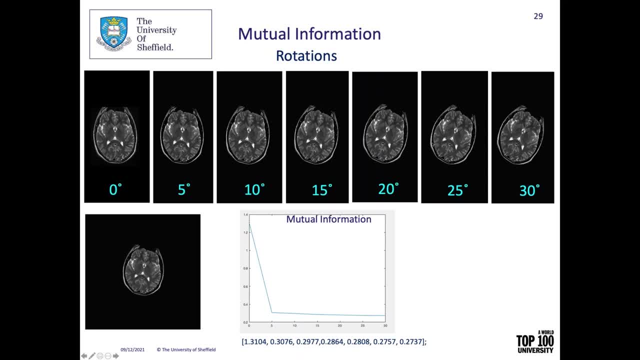 So if you have a reference image- and these are the images- at different rotations, So from five degrees to 30 degrees, If you imagine you want to register 30 degrees to zero, You imagine that at some point this the registration algorithm will rotate and map. 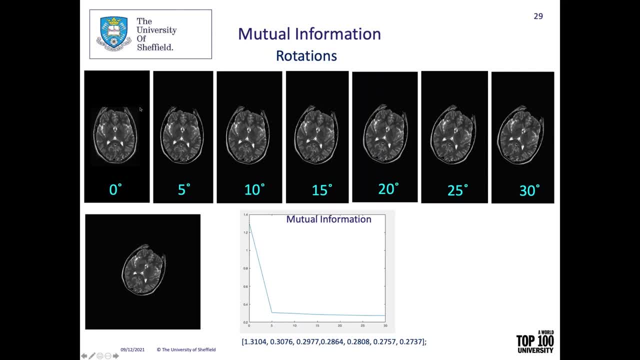 this image to the Move, the image to the fixed image. At this point the way to check the stopping criteria is looking at the mutual information which is the result of the former show before. So, as you can see here, if the two images are aligned, so zero difference in rotations. 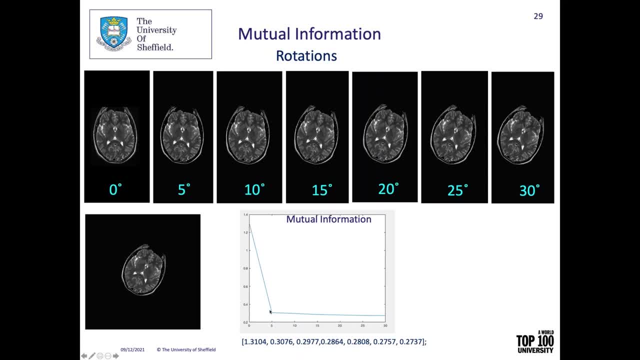 so they're perfectly registered. the mutual information is the higher The more the images are rotated, so the more are distant one from the other or from the registration. the higher is the uh, the lower is the mutual information. So the criteria is to find the maximum mutual information. 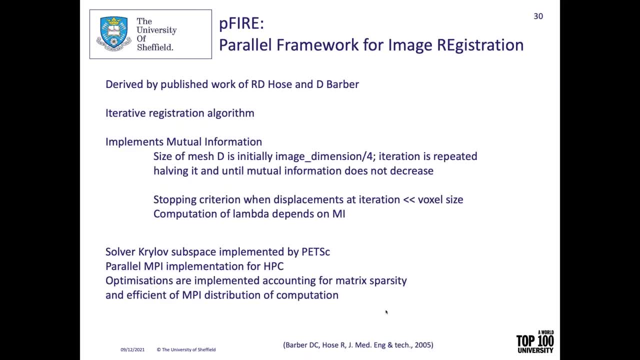 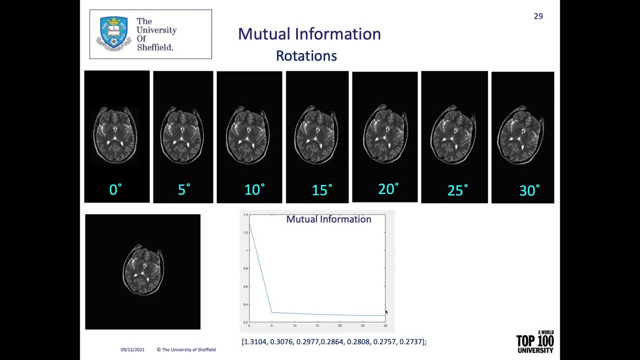 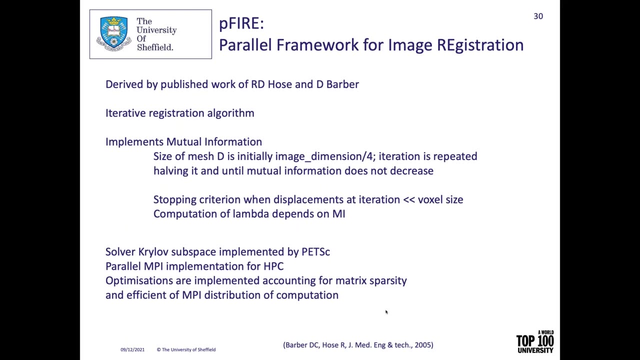 Maximum mutual information means that the image is registered. Um so, um, now let's. let's stop here. Okay, Let's talk about, uh, uh, the p-file. P-file is a software which is developed in Sheffield and is derived by, uh, some research. 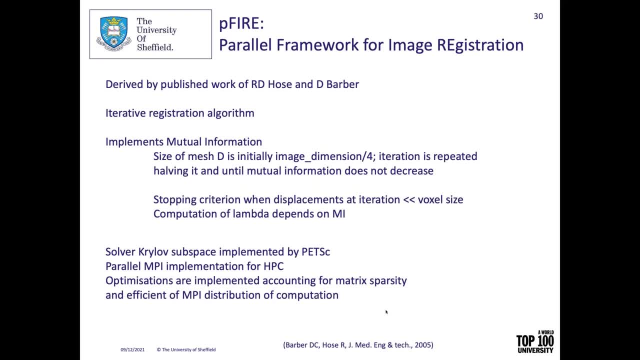 done by Rodos and David Barber. P-file implements the iterative algorithm we saw before and implements it to user using the mutual information. So in two different parts of the algorithm the mutual information is used to decide which is a stopping criteria In the uh iteration algorithm. 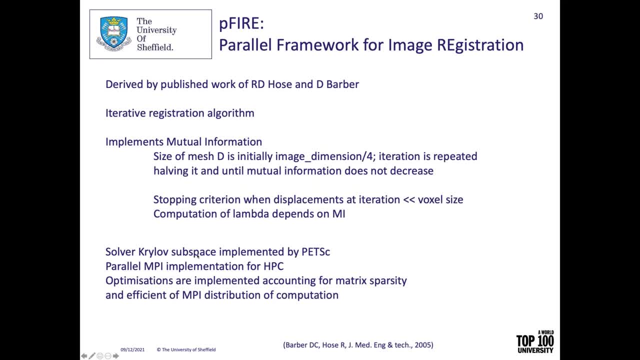 This software uses the algorithm uh, uh, the line, this software, uh. when you want to solve uh this system, uh as in uh finite element, you need to use a solver. So the A value, the degrees of freedom in the formula, the registration formula I showed. 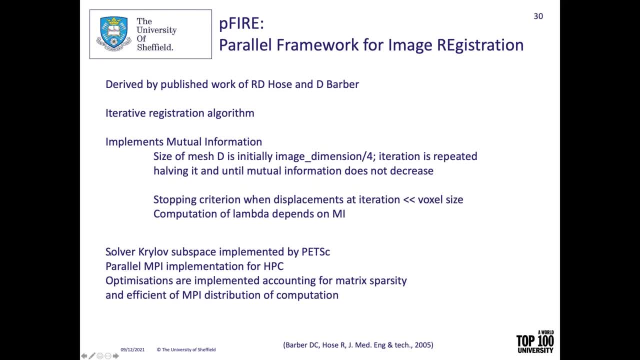 before they need to be solved. So we adopt the uh uh CRILOV solver and uh this software is developed uh with an eye. It's optimized for uh uh HPC computing. 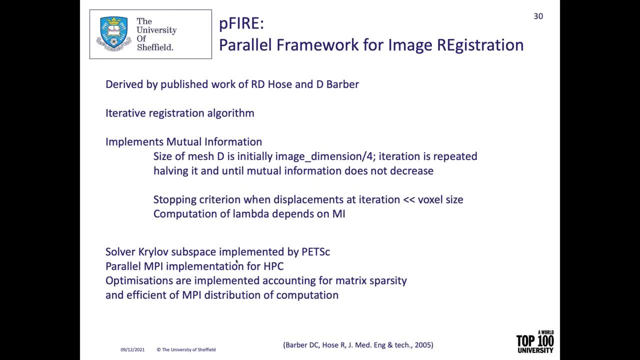 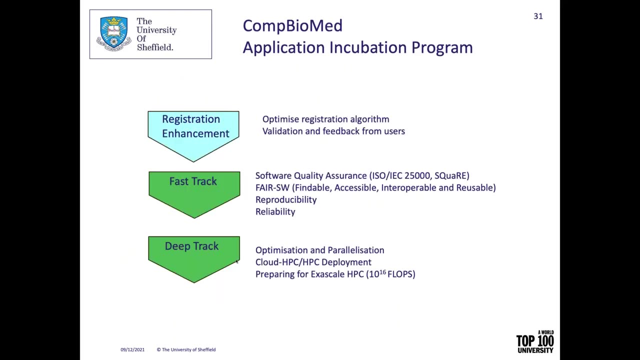 So it is uh developed in MPI And uh there are a number of uh implementation. the optimization that uh can be done and need to be accounted to uh augment the efficiency of the execution. In CombioMed we follow uh. what is the incubation um program? 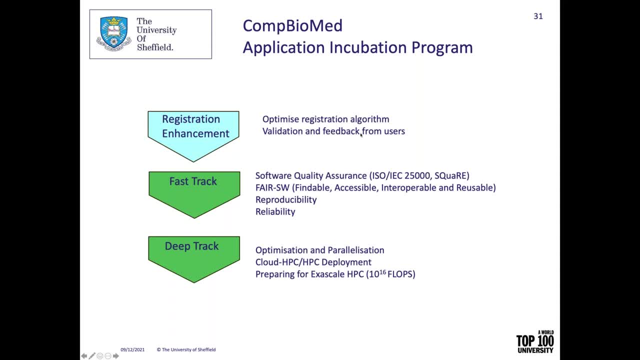 So, uh, the first step, Uh we, uh, we went through- is to try to optimize the registration algorithm and uh add uh other functionality to the original software, which is the possibility to choose uh different parameters, a different approach to register the images. 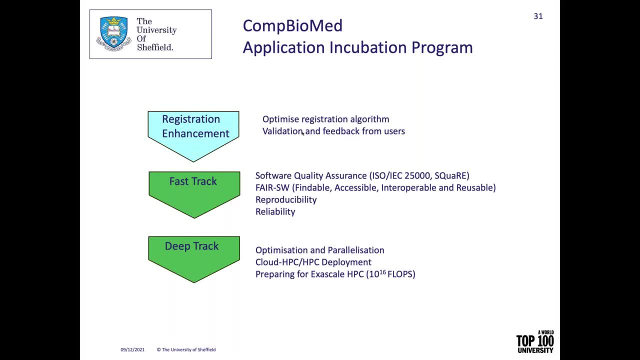 We also, uh uh recognize the importance of involving the users in this process, Uh, kind of co-design of the uh of the software. The reason behind is that, uh, um, the validation of the image is a bit further away from the. 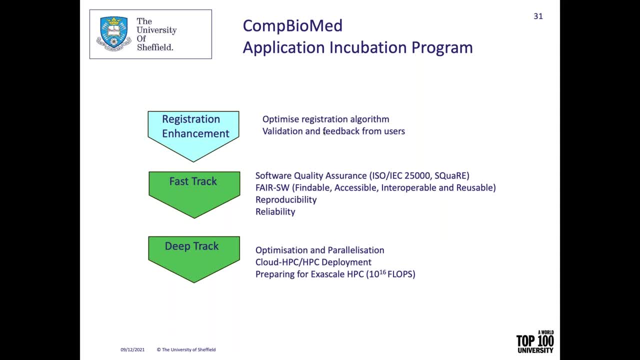 actual users. Uh uh, image is a complex matter and the eye of the expert in the field can be of high help. The second stage in this programming on Biomed is to make the software the best possible product. So we strive to fulfill all the software quality assurance criteria in the standard. 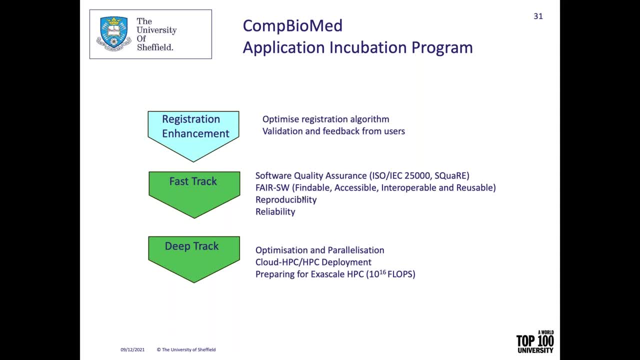 and also respect what is the FAIR software so- Findable, Accessible, Interoperable and Reusable criteria- and we want to have the software reproducible and reliable. I will show you how we dealt with this approach, so what we have done to achieve these results. 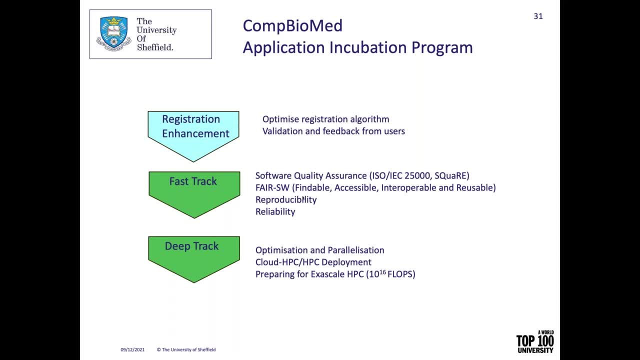 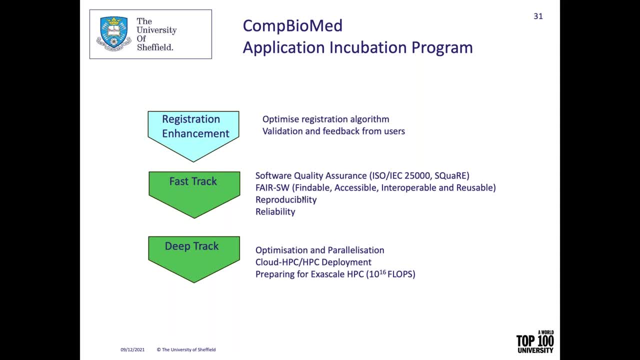 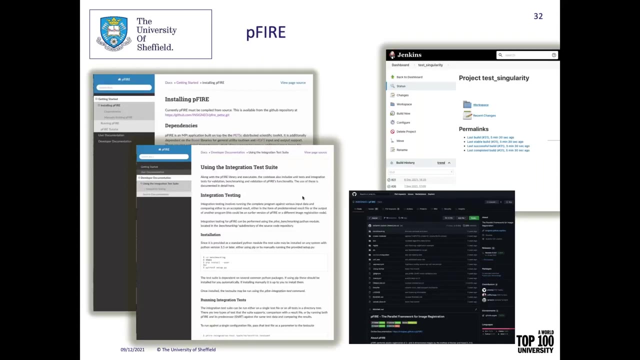 So the next stage- we already started actually- is to optimize the parallelization of the software and deploy the software on Cloud HPC. The last bit of the transaction transition will be to enable this software to run on a next-generation exascale architecture. 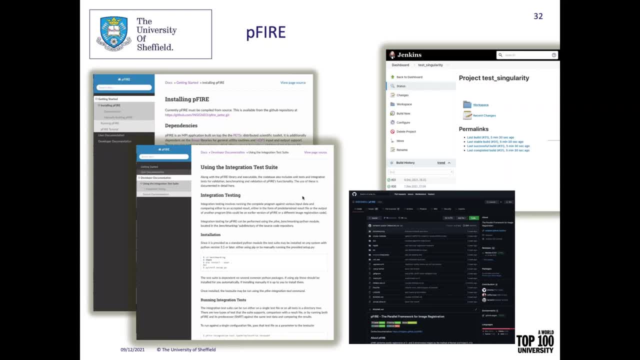 So to fulfill the requirements for the fast track, we created a set of solutions. so we offer the software on github, so it's versioned and is offered publicly with open source license. it's an apache license. then we have also the documentation which is online, and this is an 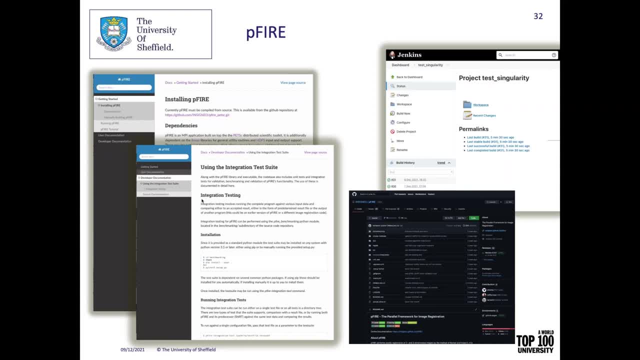 open format and is delivered through the reader, the docs standard, and then we integrate continuous testing integration. so we use the beginning travis and then we changed to jenkins because we needed to test also the mpi implementation of the software and also test the containerization that we did the fortifier. so jenkins offer more flexibility in terms of the possibility we can have. 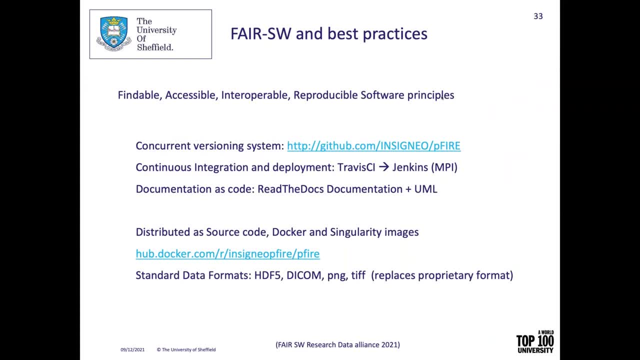 in the testing. so currently these are the reference for funding our software. you can find on github. you can just search for insignia fire. as i said before, we used jenkins replacing travis ci for condition integration deployment, so the software is written using boost test as a software continue for testing, for unit testing. 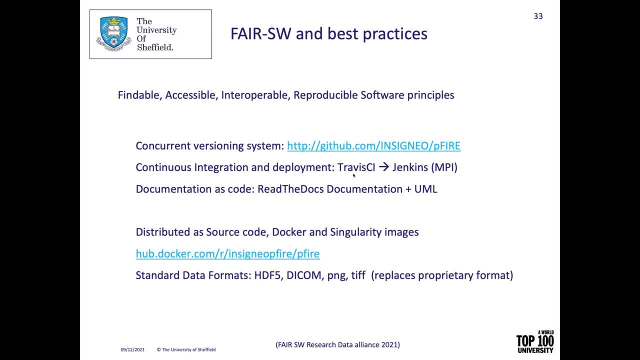 and then there is a doc developed, a benchmark, benchmark framework to test for integration and quality registration for the images. the documentation is offered through the docs and we'll be adding a second section where we have developed also the uml- um description of the software we distribute. 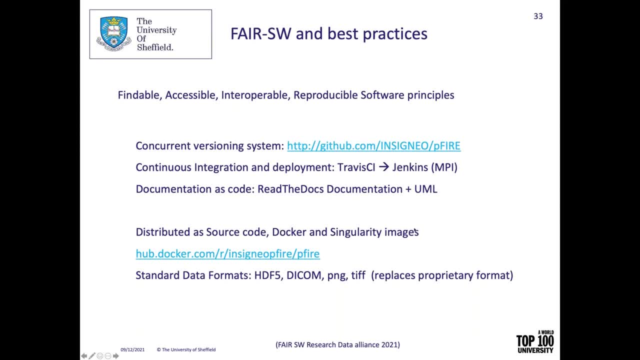 a software as a source code, but also we prepare the docker similar images. this is a requirement for two reasons: first, to allow reproducibility of the software distribute very easily, but also to involve the, the users, and have their feedback since the beginning. so we are collaborating with. 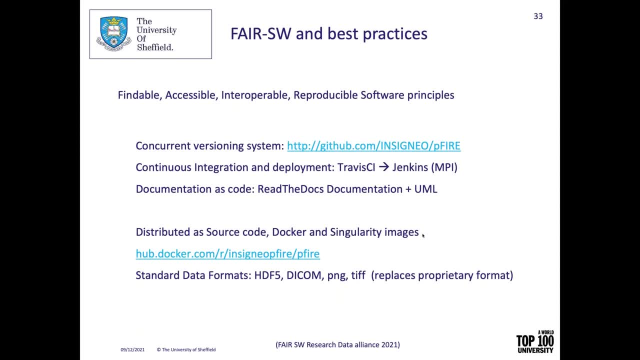 other partners in senior outside insignia. to validate the algorithm of a certain type of problems. we strive to use only standard formats. so for the images we basically use daikon, but also some of the images we can process also png, tiff and the hdf5 for the registration data and the 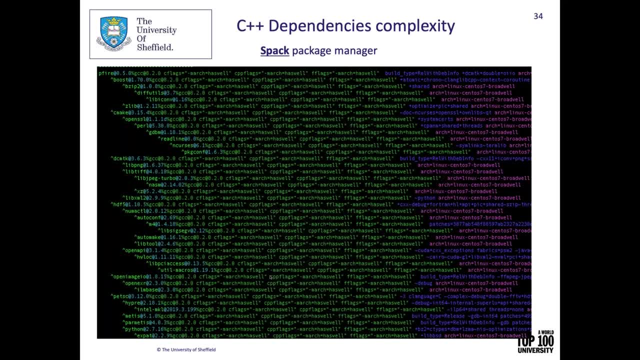 images as well. the main problem also for this type of software, the main problem is that the software does not have a lot of dependencies, as you can see here. uh, it's devastating because uh, there are, that there is a? uh, a lot of dependency, a lot of version and there are a lot of combination. 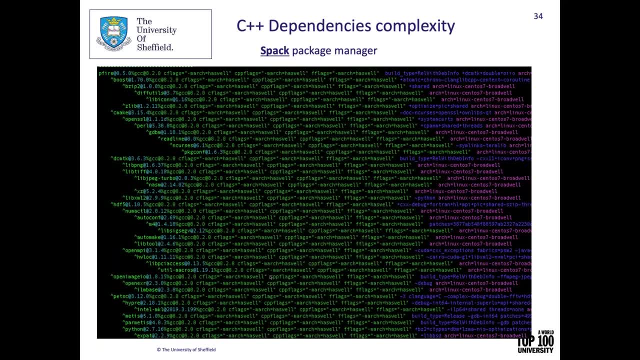 of the type of dependency that we need for pfi. we tried different package managers. we tried also spac um the all the package manager, uh, pro and cons the. the only limited application is always in the goodness and the woodwilling of the maintainer to maintain proper. 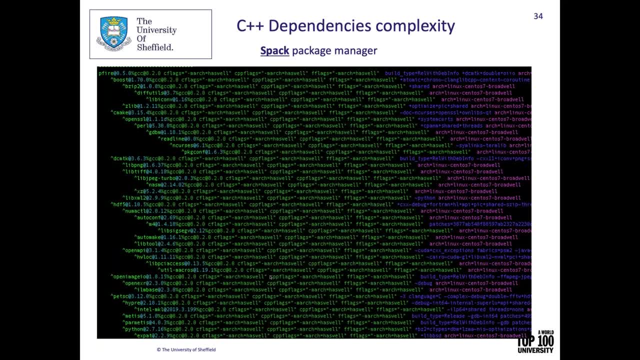 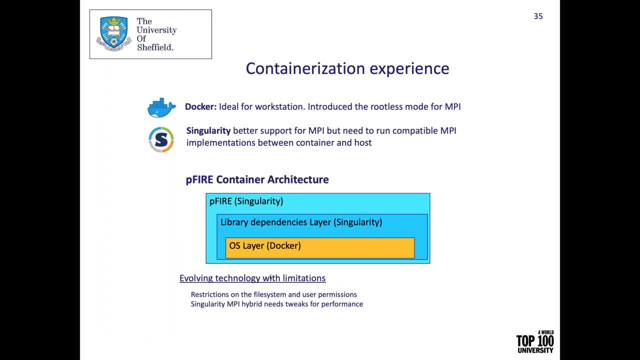 uh package manager to allow to install them. do not have problems. so our containerization experience is: uh, we initially use docker, but docker is uh the best solution, in my opinion, for workstation. and there was a problem. uh, it's a ever-changing uh scenario. it changes uh continuously every month, but when we started, there was a problem that 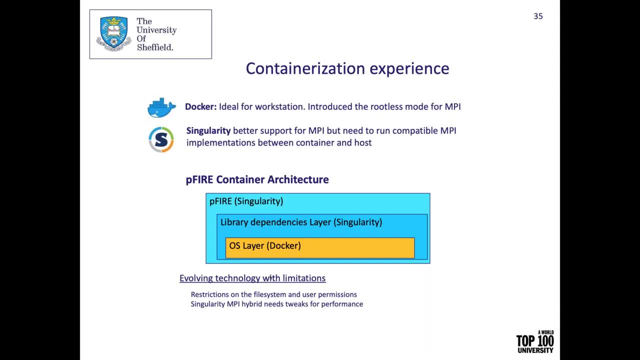 you. you can't use the root user for a running mpi, while with docker you needed to use the, the root user. now they introduce also the root rootless mode, so that could be solved that problem. we then moved to a singularity which can reuse what we've done with docker. 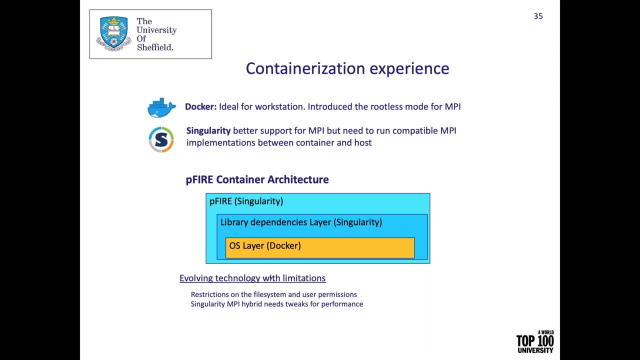 and uh. the main reason is that uh singularity supports uh has a better support for mpi, so it's been developed within having in mind uh. hpc, hpc solutions, um, all these softwares, uh can consume something strange. but this concept of containers, containerization, is quite old. someone can remind. 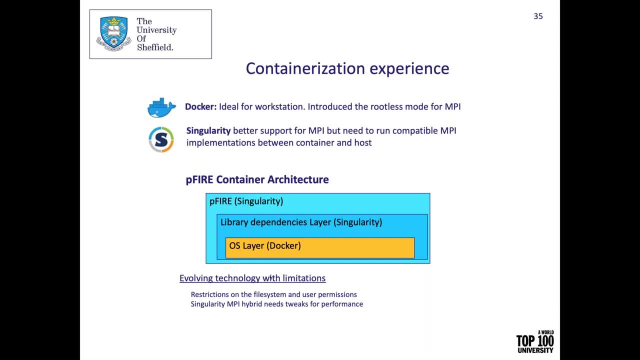 ch root linux containers is more or less the same concept. that is evaluated in time, but the basic concept is the same. the problem we had in developing these containers is that there are a lot of dependencies and it's complex to generate from scratch, takes a lot of time to generate from. 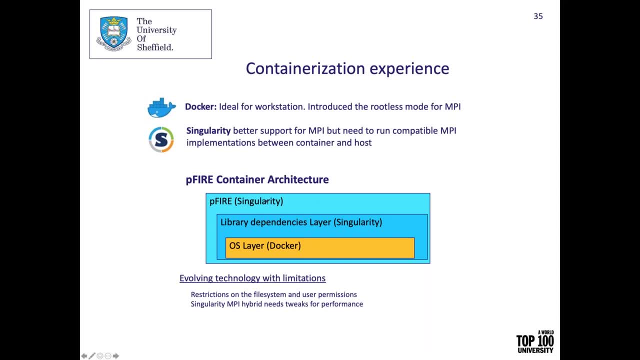 scratch all the software, so from including, from profile, plus all the dependency and the operating system. so what we did is to decouple the three layers so we have the os layer, which is a container. it is included then in another container. so once you've once you've generated this container, there is no computational requirement for generating the. 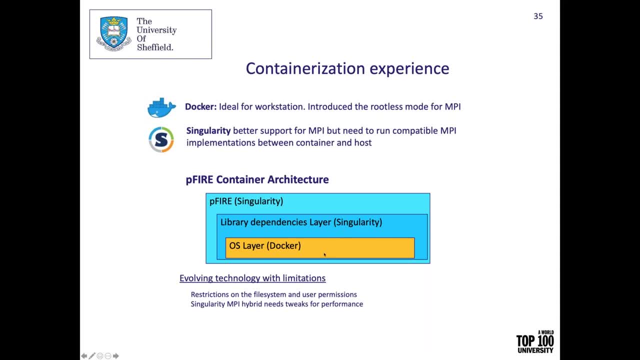 the other one, the library dependency container, which include this one. so once you generate the library dependency container, you can include this one, the following one, so there is no computational effort to generate this part and you just generate the container for p5. the good thing about this approach is that you can have a several version of these layers. 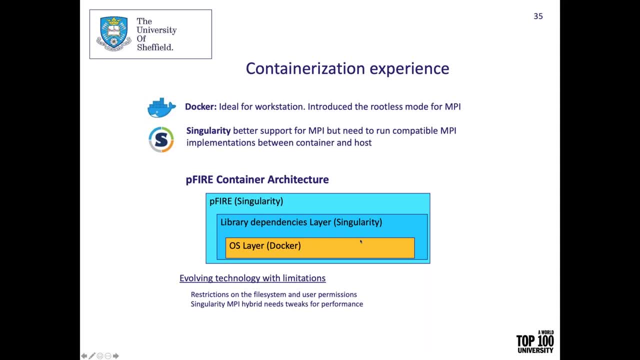 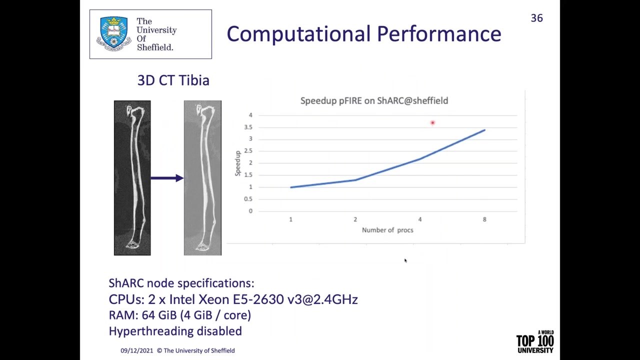 with different version of libraries, different version of operating systems, and you can have a matrix of combination and test all of them in the continuous integration system. these are all evolving technologies, with the limitations and the problems are always behind the corner. we started to test the performance of the fire and, in this case, uh, the daily test we did. 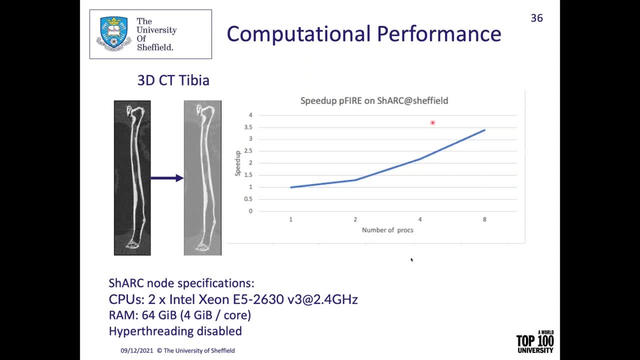 they were on small-scale images and the speedup looks promising, but it was only on a subset of the, on a small case. It didn't. we didn't end up. we didn't end up using more memory than the one that was required by a single node. 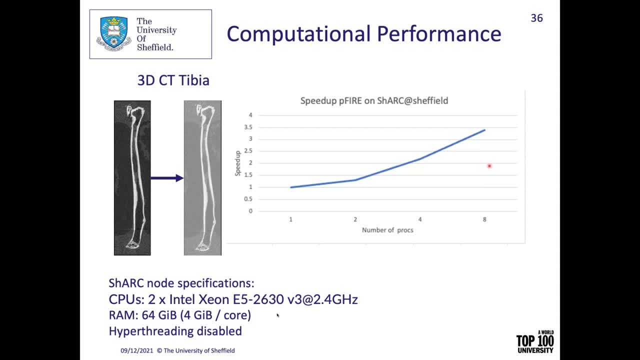 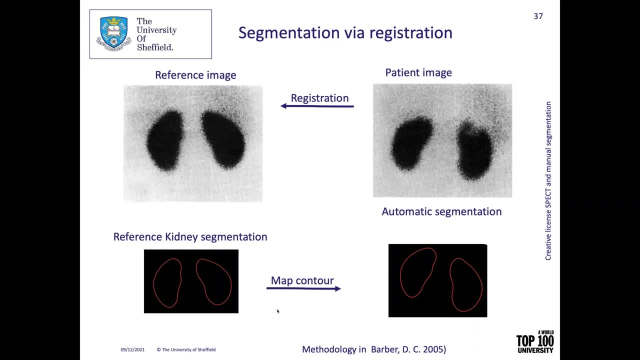 so we used maximum 64 gigabyte on a node of two Intel Xeons. So the registration is not just a process to register two images one to the other. There is another interesting application of this. So assume that you have. this is a kidney renogram. 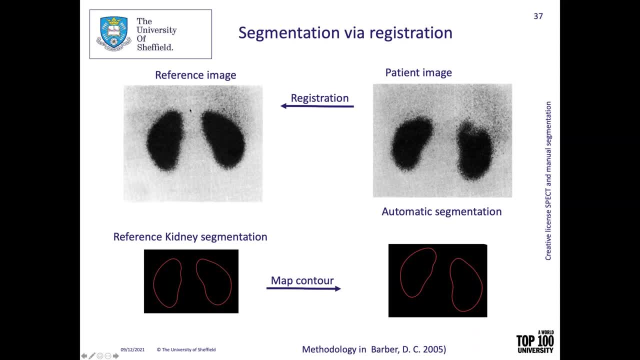 so it's a scintigraphy image. Let's say you have a reference image and a patient image. One of the problem in some assessment of patient health would be important to segment, to trace the boundary around the image. So let's assume, imagine that you have an oncology patient. 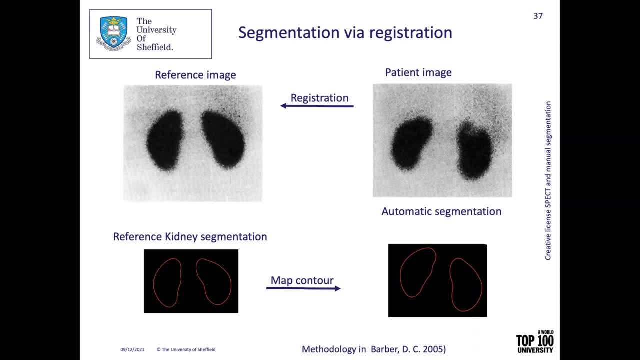 and you want to understand if the volume of the cancer is growing. So you need to find a way to trace the boundary, to segment the organ or, in that case, the cancer, and in time, with different, with new images, you want to do a scan of the patient. 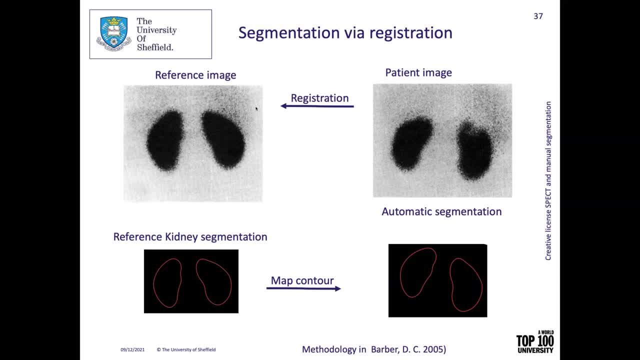 You want to compare, realign the images and compare the sides of the tumor. In this case we're talking about the kidney. So we have a reference patient. We can find the best. the golden say. assume that this is the golden standard. 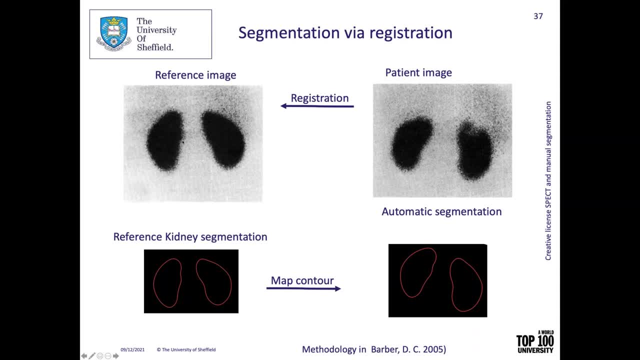 to segment this kidney. So then comes a new patient or a patient at a different time step. This is the following: scan What you will do if you want to segment again this one. It could be a different operator doing again manually, So it will introduce error. 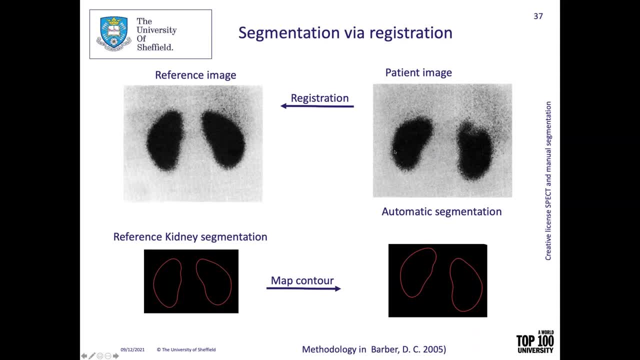 One of the solution could be to take this image register to this one, use the mapping function to apply to the golden standard contour golden standard segmentation and then transform this segmentation to the one of the patient image. So just computing the mapping. 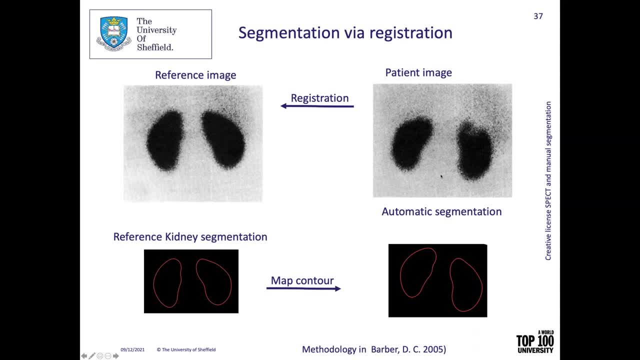 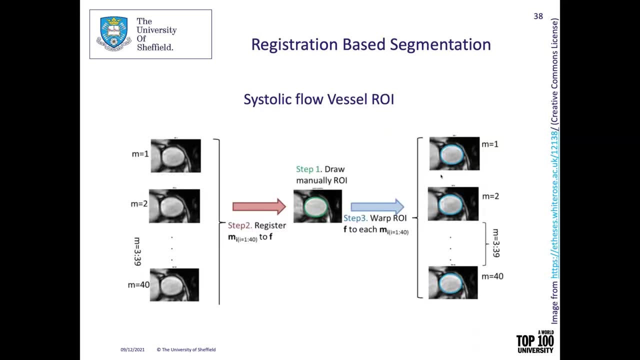 you can then reapply the segmentation to the new one and you will have the segmentation for free, without, let's say, operator errors. This is another application. You can find the full description on this PhD thesis, the Angelo Longo of Angelo Longo. 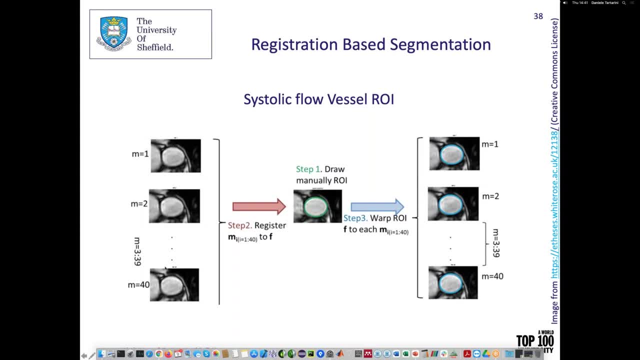 So this is a section of a vessel and this is a series of images taken in 40 time steps. So heart is beating, the vessel changes size and you want to know how much the size is changing, So you need to measure some parameters. 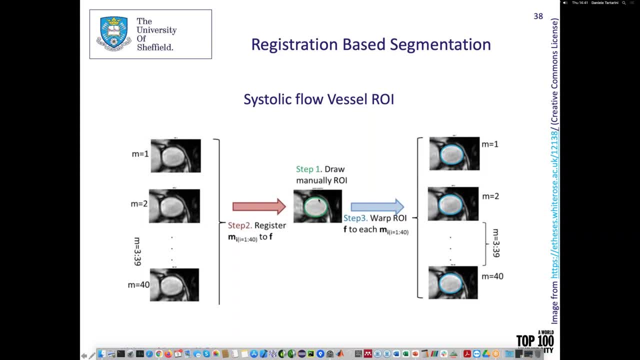 So what you can do is to segment the first image And then, in time, when you have another scan with another sequence of image, you can register the new image to the moved image, to the patient image, and then transfer the segmentation. So it applies in two different ways. 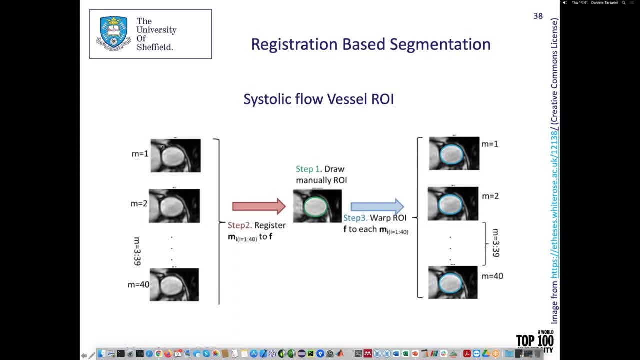 The first one is you can just segment the first. You can consider the first time step as the reference image, Segment it and then register the next And then the next time step to the fixed image and apply the mapping to segment the second one. 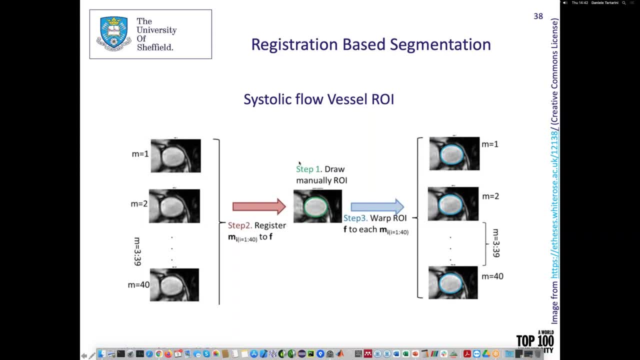 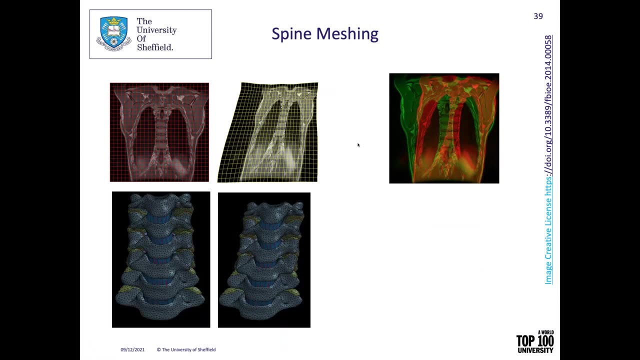 Or you can do the same work for a different sequence, taken in time or during another session with the patient, Another application. you can use the same method to transfer and you can use the big measure that I used to model the component part of the body. 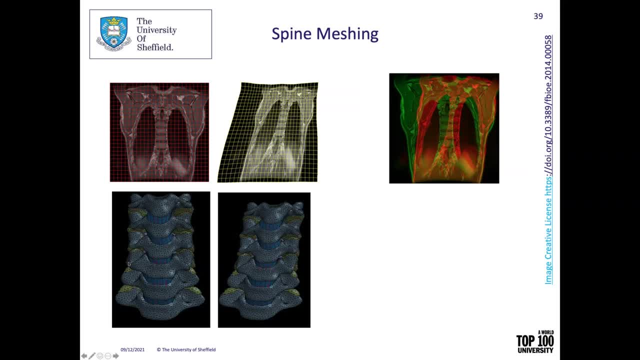 In this case, it's assuming that you have a finite element model or any type of modeling that requires discretization of the, in this case the bone. This is the spine, So it's the same problem that applies. You can find a way. 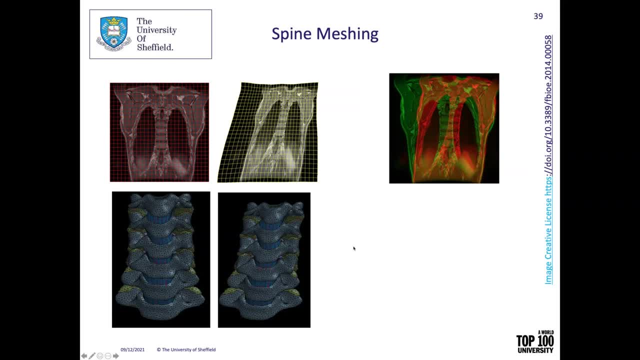 There are a few works done by different groups, including ROAD-OSV, on the vascular charge system, but you can see them, You can identify the bone, the internal bone, the limb, and after being able to do the sequence, and then you can just go on and see anything. 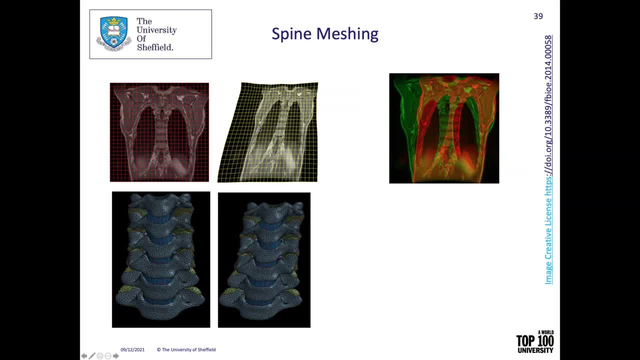 register the two images, find the mapping between the two images, so the registration mapping, and apply the same registration mapping to the mesh. so if you have for the reference image the optimal mesh describing this case, the spine for every other patient or every other time step later, you can just register the new image, new patient image, to the reference one. 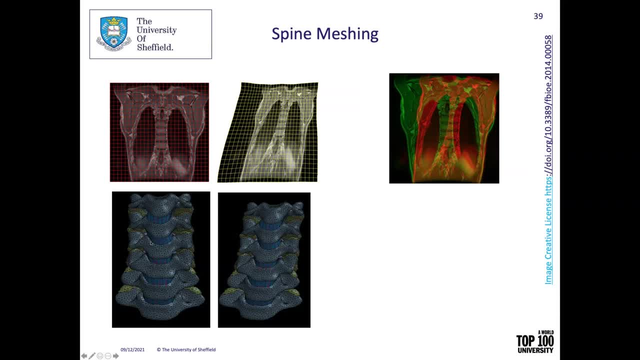 and applying this mapping, you can just obtain the correct version for the new patient of the mesh. this is an artificial image to associate qualitatively these two, these two. one, there is no work. uh, associated with this one is to explain, um, how it works. there's plenty. 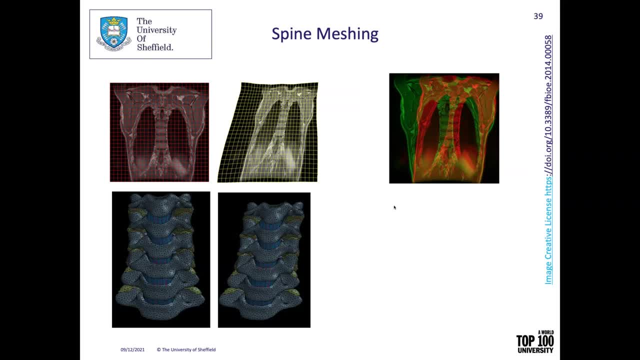 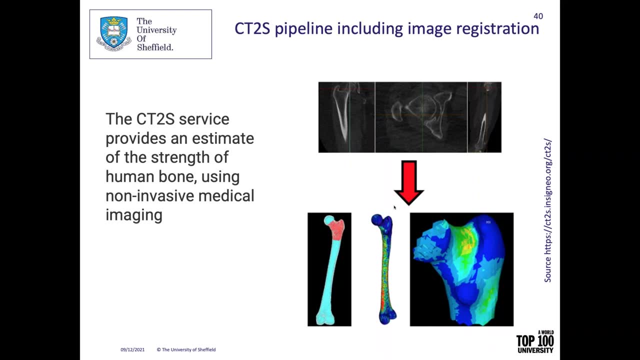 of other papers but cannot be used for, uh, copyright reason here. another application is related to the um- biomechanical properties of the bones. so the ct2s service what does is to take two scan of the same bone, one in a relaxed scenario, another one subject to attention. you will have two different images. if you register the two images, you will. 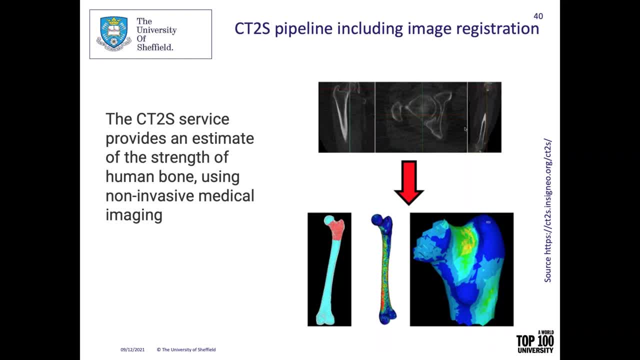 find the displacement, the registration function. but the registration function is just the displacement. so this data that you have, you can convert it and obtain this, the stress strain you need for the bone. so this is used by uh one group in uh sheffield, led by uh ricardo lara, to uh assess the, the strength of the bones and the probability of fracture. 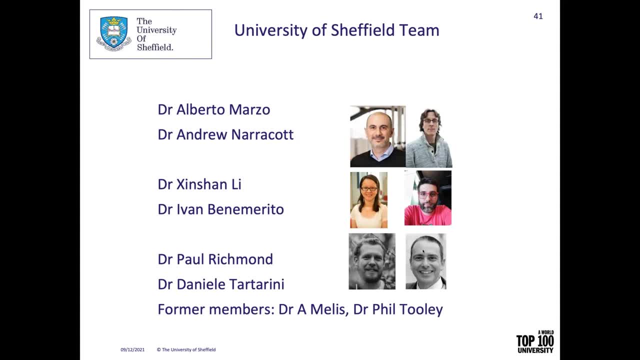 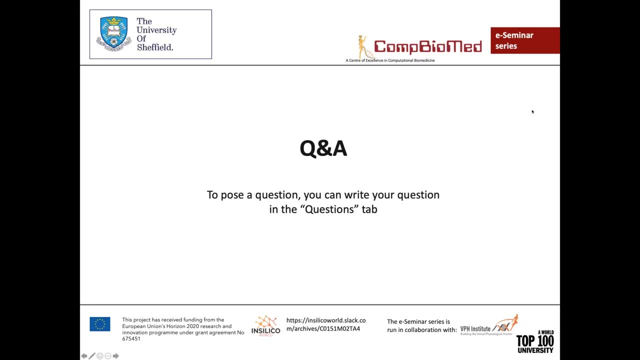 so i would like to thank all the all the group for uh the contribution to the the work, and this is the team in sheffield and i'll leave you the floor for question. fantastic, thank you very much, daniel. just a quick reminder for the audience, if you have. 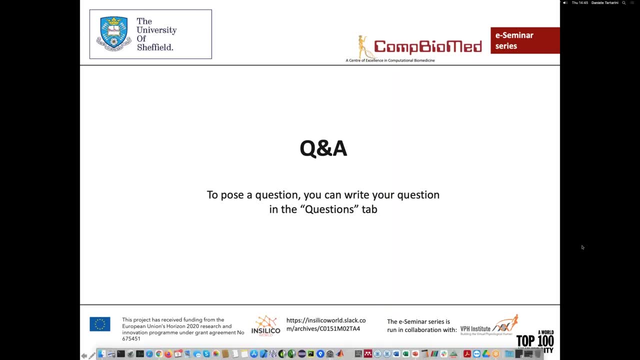 any questions, then please go ahead and write them in the questions tab so that i can read them out for you. now, whilst we wait for the questions to start coming in, i've actually got a couple of my own for you, so i'll leave the questions for you, and then i'll just give you a. 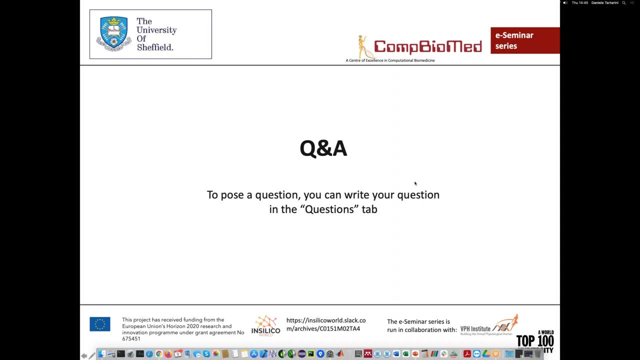 for you. So in the presentation you mentioned a few times that this theory scales quite easily to three dimensions right, And we kind of saw a little bit with the spine reconstruction there. So has this technique been successfully applied in the three dimensional case And 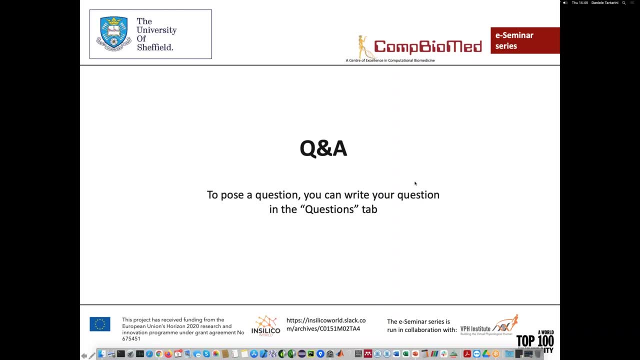 how big an impact is there on the computational resource to perform image registration in the three dimensions? Yep, So far our software has been developed for 2D. The 3D version is under validation And the theory applies is the same. It doesn't. 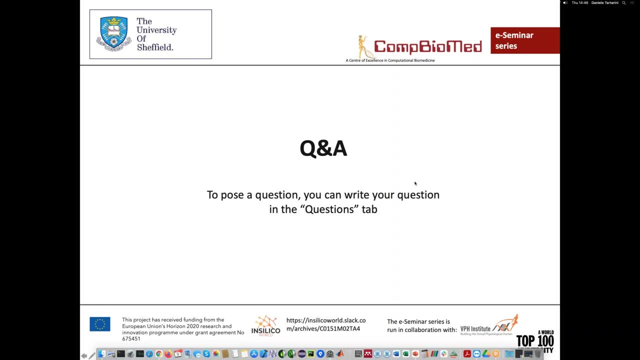 change the formulation of the theory. So what you can see for the 2D images can be applied for the 3D images. The complexities in the pre-processing and post-processing that you need to apply for the 3D images. Let's say, for example, if you have a DICOM image that is not organized properly with 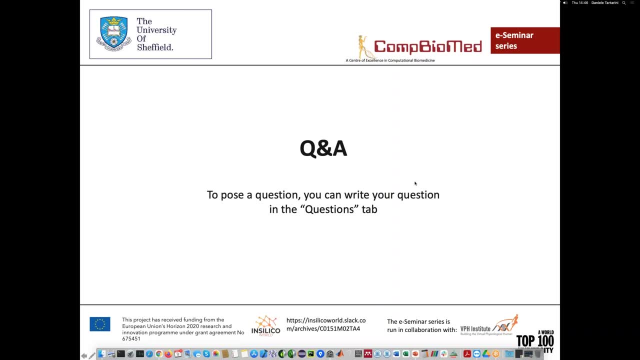 all the scans, you need to find a way to organize the volume of data. So it is just a processing problem. Theoretically it can be applied And it has been applied successfully. There are a few papers that has been published of other version of this theory applied before. 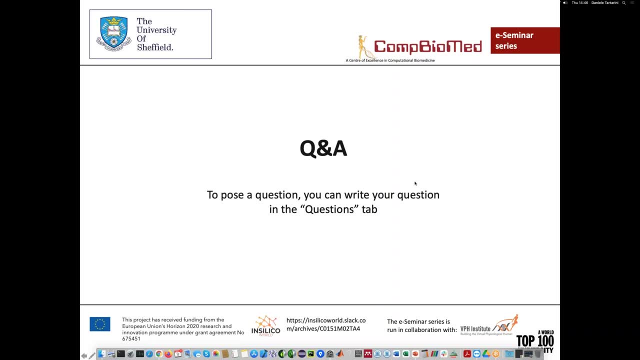 So this theory has been developed by in Sheffield, by all those that they've barred. they've been barred And there is different papers describing this application, even in 3D. P5 is inspired by this theory and is an implementation of this theory from the papers: 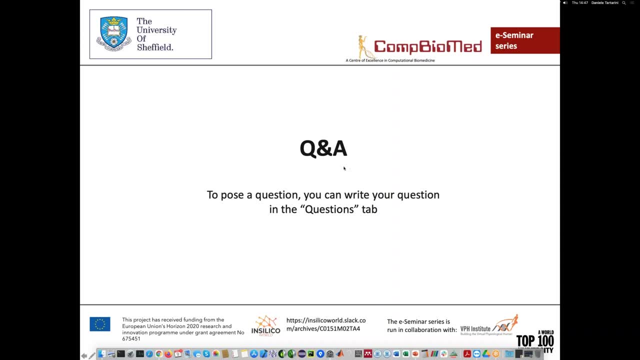 Right, I see, Thank you. I guess it seems mandatory at this point that I ask something with regard to the Exascale. So what is the current state on the path to Exascale here, And do you plan to use any GPU computers? 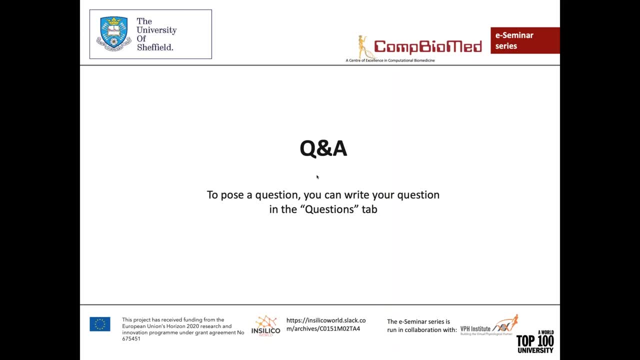 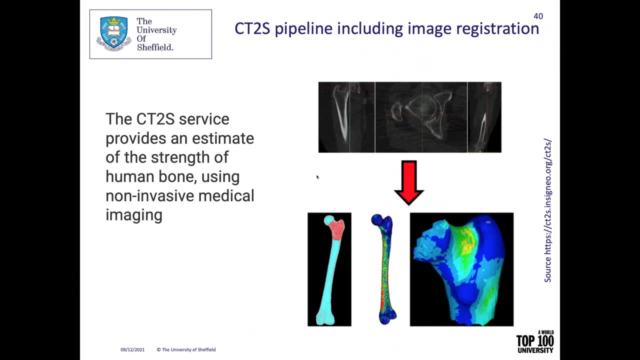 So we have in mind. so this service here is a micro CT is based on micro CT images And they use the images from the diamond source light And these images are really heavy So they require tremendous computational power. So we are talking that each time step can. 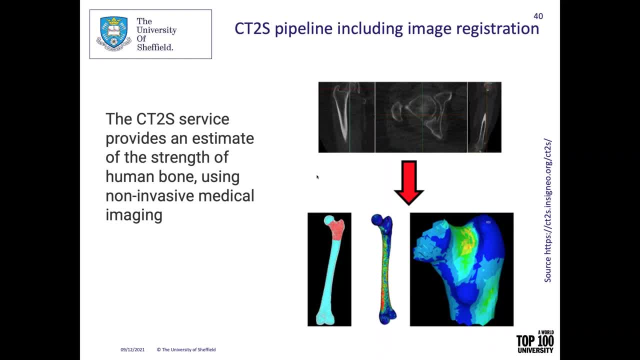 be in the order of tens of gigabytes. So the problem is that you need to, Okay, Okay. So you need to allocate enough memory and you have enough power- computing power capacity- to solve the problem, Being a finite element problem, and the solution is about solving. 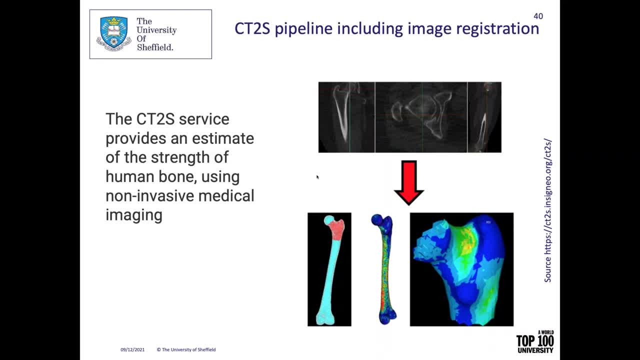 matrix vector products. So generally, in the worst case scenario, there is an interesting accelerations of using GPUs with respect to CPUs. The thumb figure is that one order magnitude. So, moving to GPUs, The complexity is always to find the right optimization, a combination of settings to 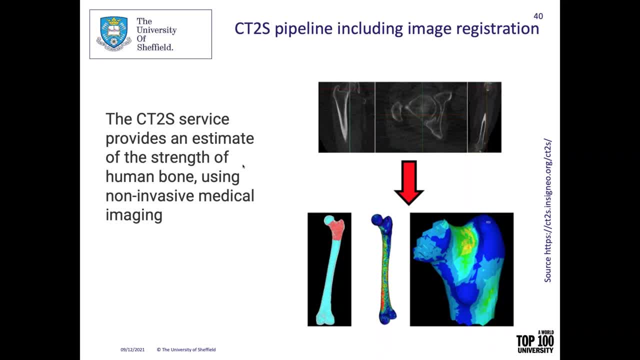 formulate the problem the right way to be run on GPUs. We haven't tried yet. The libraries we rely on let's see they have solvers implemented already in GPU. So this is some work we would like to do in the future but we haven't done yet. 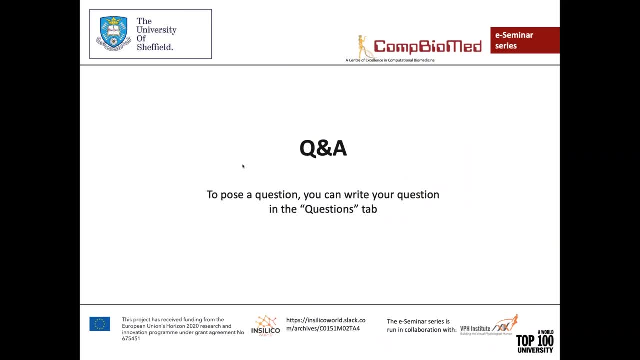 Sure, Thank you for that. I haven't seen any questions coming from the audience yet, So suppose I'll ask another one. and this isn't really fully formed in my head, I suppose, but it seems as though this technique is very much reliant on having a high quality target. 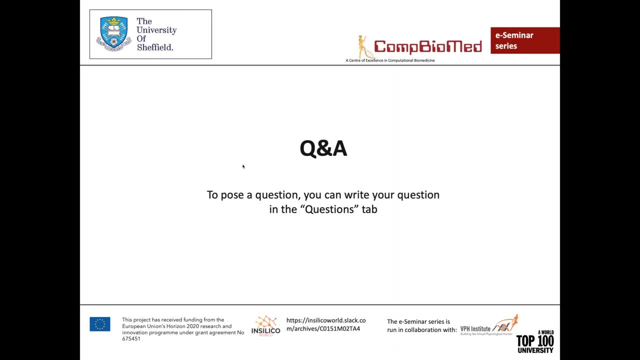 image right? Is it always feasible that that can be attained? How do you assess whether or not your target is? It really depends on the problem. So if you imagine that, what is the pipeline? So you have some scanner that acquire information. This information depends on the technology. 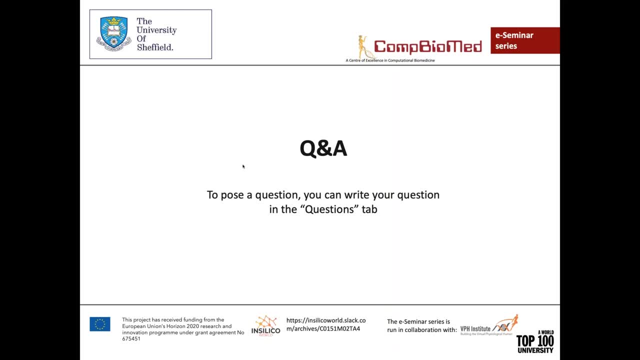 used. So there is some limitation in the resolution of the of the problem itself, in the physical problem. Then this machine- they have a limitation in their own resolution, So it depends on the resolution And then you process and you apply your solution to your methodologies. 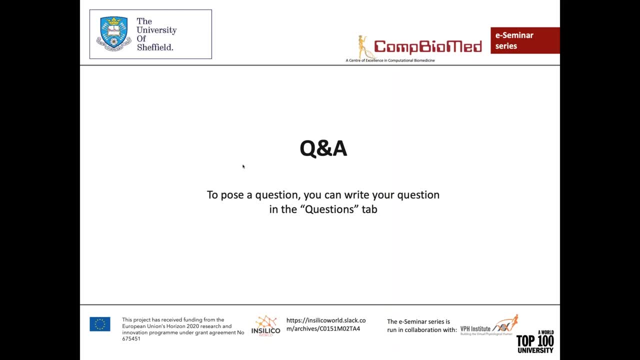 to these images And then you show these results on screens which they have another type of resolutions. So there is the first problem, which is the transfer information between in this pipeline, And you need to take into account what are the resolution of the different 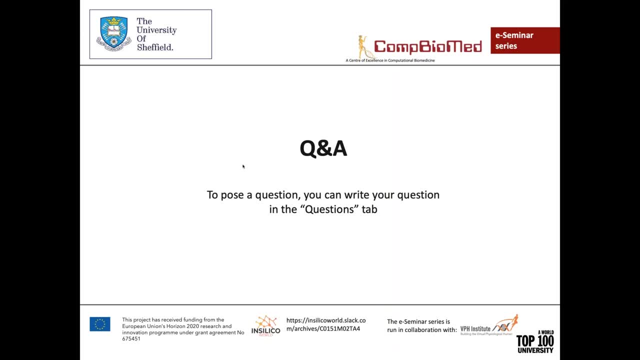 stages, Assuming that everything is fine. the other problem: you have the maximum combination of resolution to obtain the right resolution to make the assessment, because that's what is important. The other problem with this approach is that the equation has been there is a tiller series. 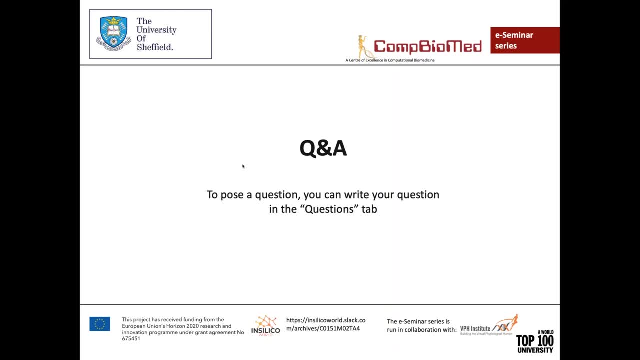 inside the equation. So that includes some generation of error that has to be assessed. So to overcome this one. I found it quite complicated to validate these algorithms- not this one but in general the registration algorithm on images- because different images of different organs and with different modalities have different, let's say, resolution. 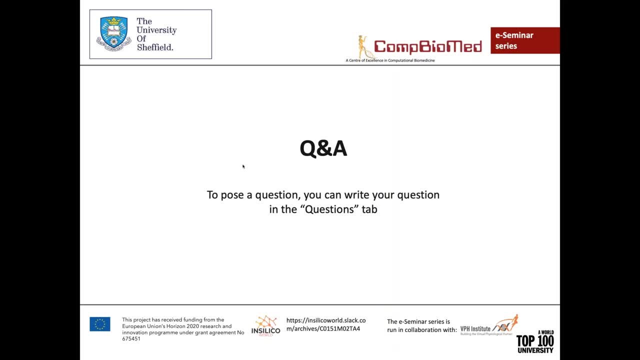 Or meaningful resolutions, and it's difficult to compare one algorithm to the other one. So one thing we have in mind is to adopt use some validation data sets that has been used in the public competition to compare the different approaches, and one approach could be also to insert inside the images. 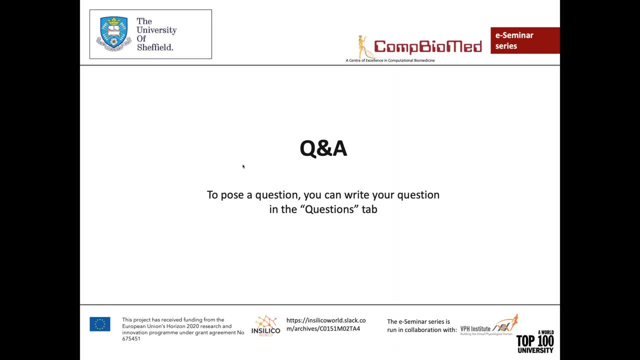 So use some data, set where has been inserted the crucial points, Insert the images and then compare with the results to check if the registration is correct considering the crucial points. So I hope that answered your curiosity. Yeah, it certainly does. Thank you. 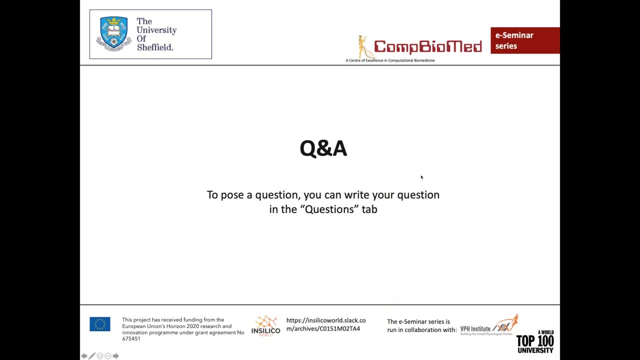 I still haven't got any questions from the audience, I'm afraid. So I'll ask you one more, and after that, if nothing else has come in, then I'll wrap the the session to a close. But in principle, these image registration techniques are they? they seem to be kind. 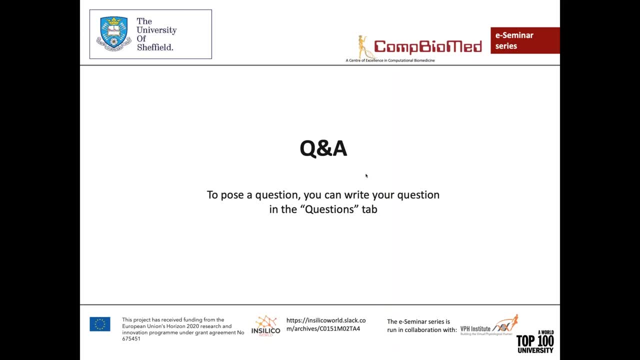 of agnostic right to the underlying hardware. So, in that sense, could these techniques be extended outside the medical domain, you know, for example, to processing astronomical images from telescopes, just as an example? Indeed, I'm not familiar with this type of images. 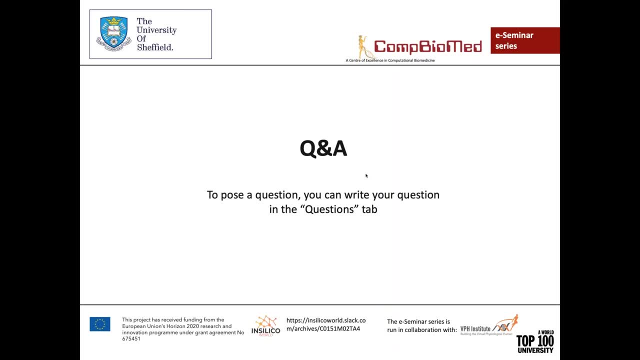 And I can tell you that this approach is used, for example, in fracture, so in civil engineering. So it's called the digital image correlation You can have. You can analyze the picture of, let's see concrete under stress and then fracture. 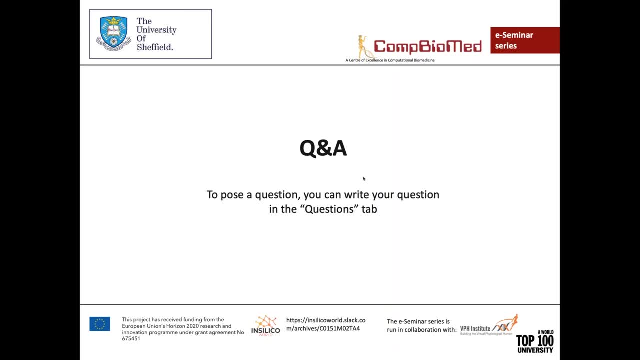 You can use the registration to assess the stress that this piece of cement has been subject to. So this is another application. This is a registration. You were asking for the Those images regarding the Not segmentation, just for the registration right. 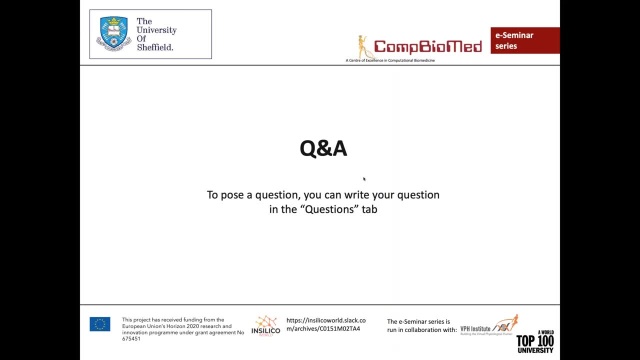 Yes, indeed, So usually, if I have in mind the image with the stars, for example, you can imagine this image as a series of Gaussian functions. Okay, Okay, The complexity of registering is that if these are to distance, there could be a problem. 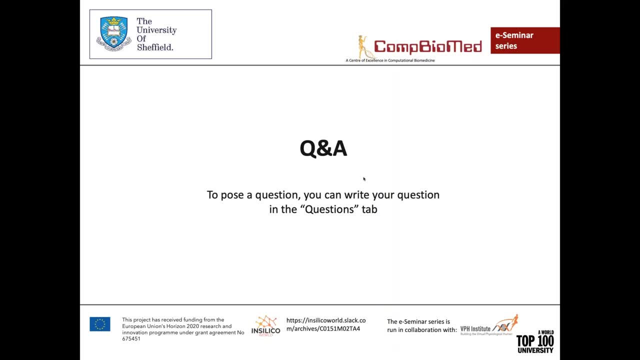 generated by the fact that there is a theory of series underneath these algorithms. So if they are to distance and the shape of this function is not smooth enough, you can have some conditioning in the problem that you will not want to achieve the results you want. 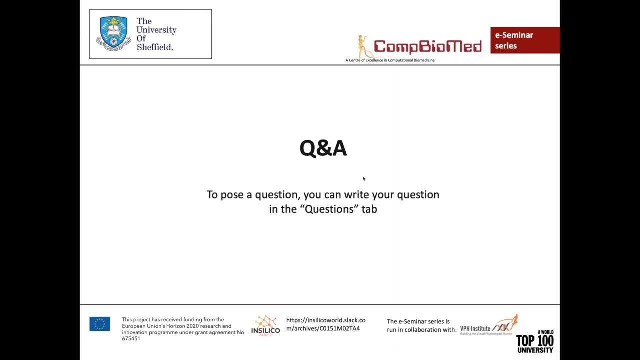 So it needs to be tested And I simplified the presentation. but there are different parameters of smoothing that can be used and changed and some kind of introduction of memory inside the solution of the iterative solutions. So the algorithm need to, I would say, tailor to different type of images. 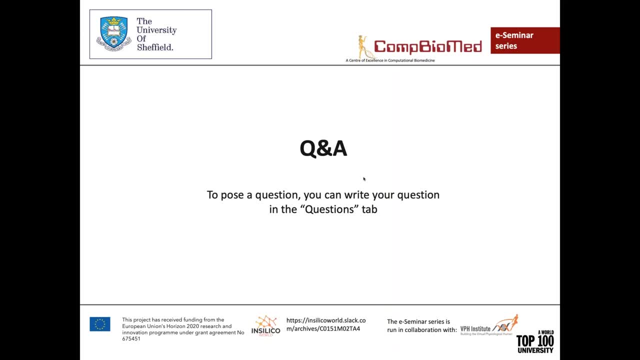 And then that, I think, is the difficulty to translate on different domain. Even within the biomedical one, you can have a different type. For example, if you have a section of a bone, it would be different from having a transverse section of a bone. 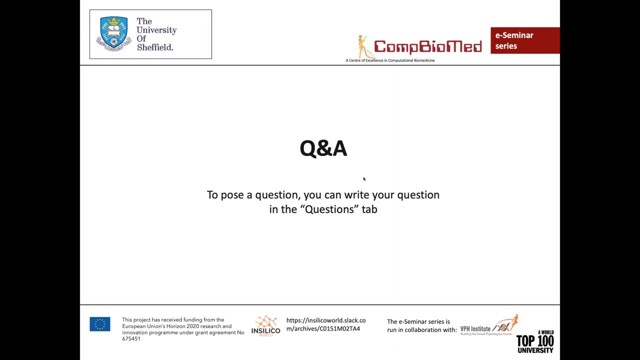 So if you take a leg, it would be easy to register a cross-section with respect to a longitudinal section. But with the proper changes in setting the algorithm, you can achieve both. Sure, I understand, I understand. Well, those are all of the questions that I had for you. 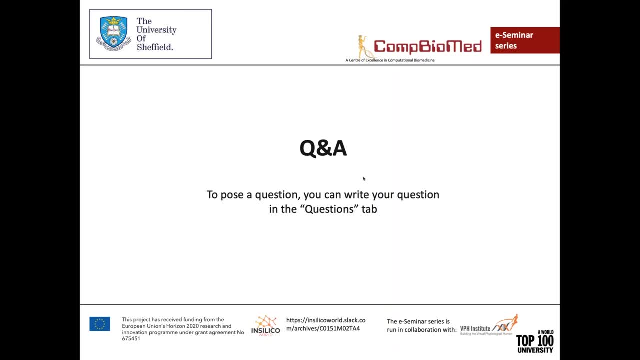 Have a good day. Bye, Bye. You haven't been any more from the audience, So thank you very much for giving such comprehensive answers to those. I very much enjoyed the talk. So thank you once again, Daniele, for giving us your time today to speak about biomedical.